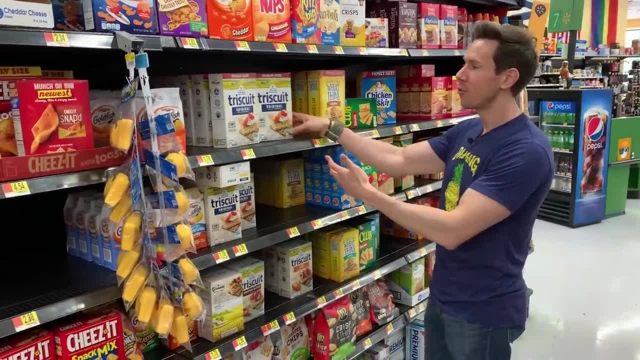 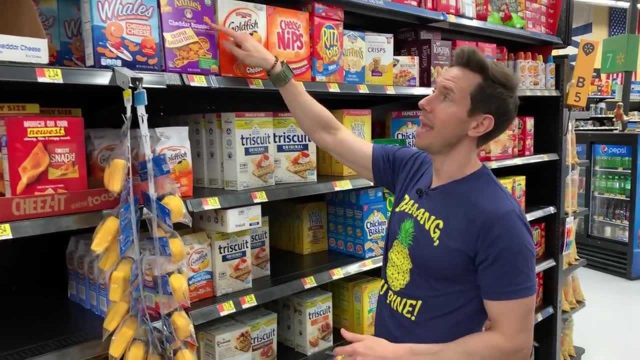 crackers really quickly. So many of these are just garbage. Even Triscuit. it has three ingredients. Whole grain wheat is one of them, but they're using processed canola oil. Best in class here is going to be Annie's organic cheddar bunnies. Organic cheddar cheese. organic dairy is the best, but there is a better. 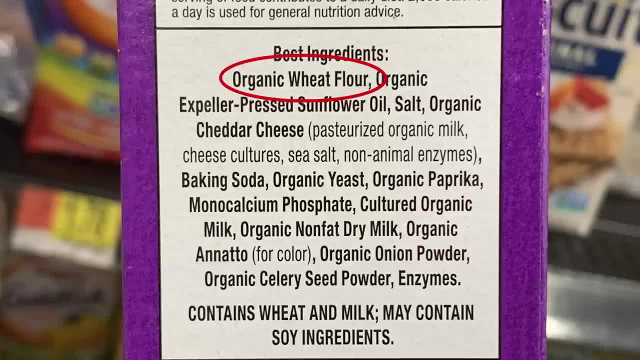 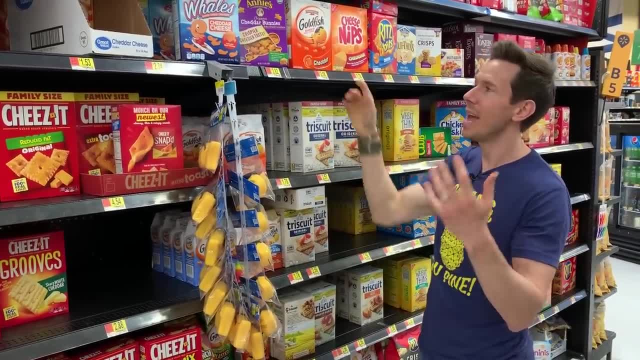 one at Whole Foods, because look at the first ingredient: organic wheat flour. It's not whole wheat flour. Always look for whole wheat and whole grains because it's a complex carbohydrate. It's not stripped down to the endosperm or their simple carbohydrate. That's the best here, but we can do. 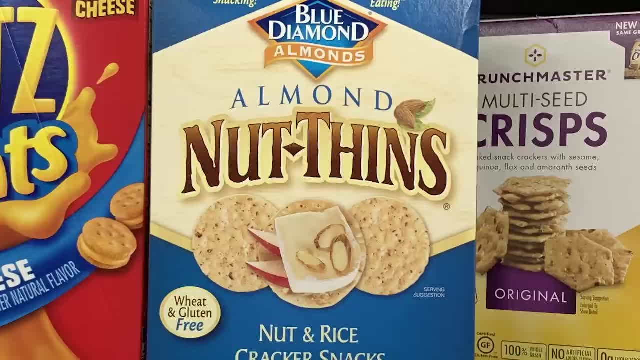 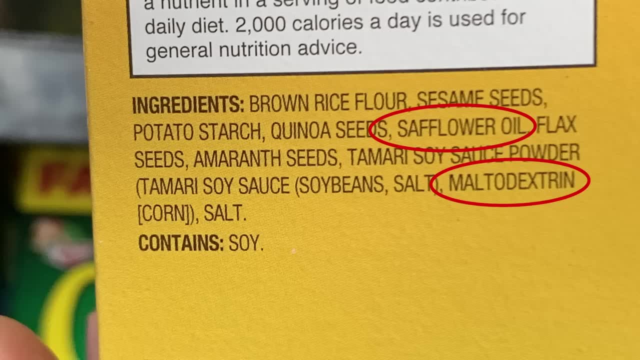 better, And then stuff like this looks really good. It's a gluten-free nut-thin cracker, but they use natural flavorings. This is a multi-seed crisp, and then everything's good until they use maltodextrin, which is a food preservative. that's very bad for your stomach, I'd say. the best thing here is 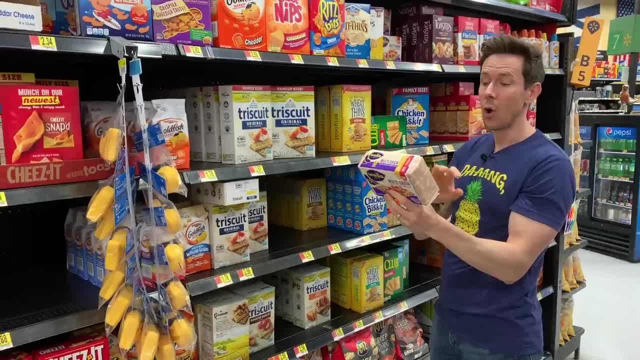 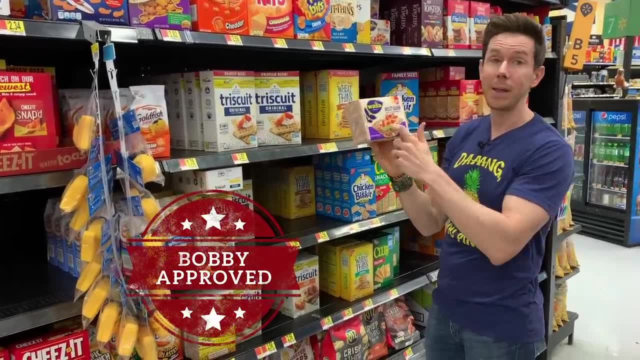 actually old school wasa crackers. You guys look at the ingredients: Whole grain, everything super clean. I know it's not the most exciting crisp or the most exciting cracker for your kid, but here at Walmart this is best in class. Now let's get out of here. 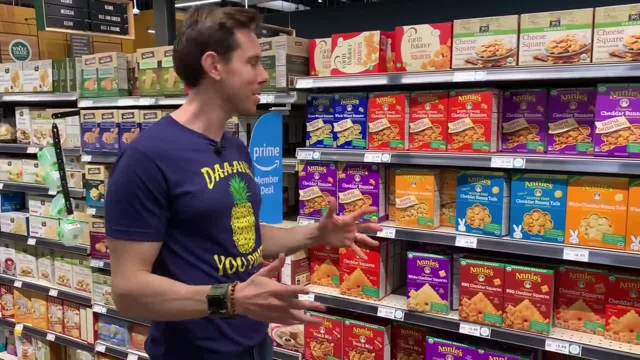 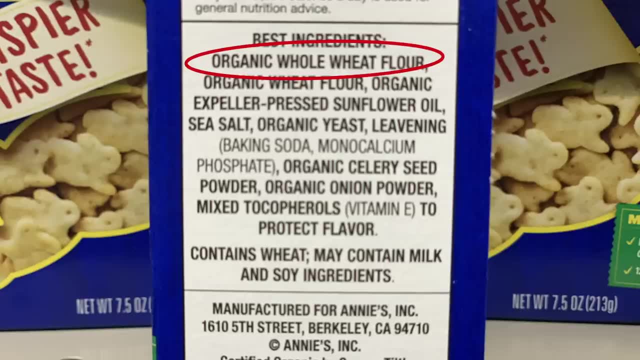 All right, Friends, this is pretty much the only cracker I can do. a Bobby approval on Annie's Whole Wheat Bunnies. Why Look at the ingredients? It starts with whole wheat, Super important to meeting whole grains. It really satiates your hunger. It doesn't spike your blood sugar. Expeller-pressed sunflower. 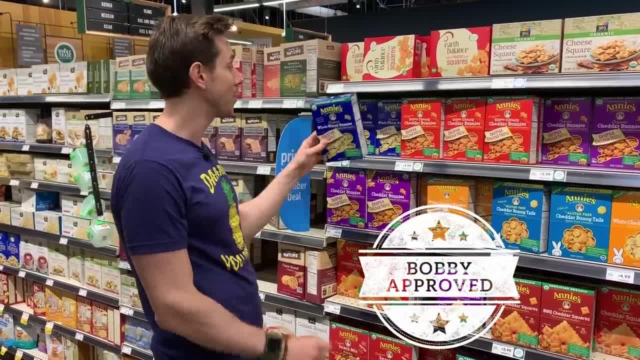 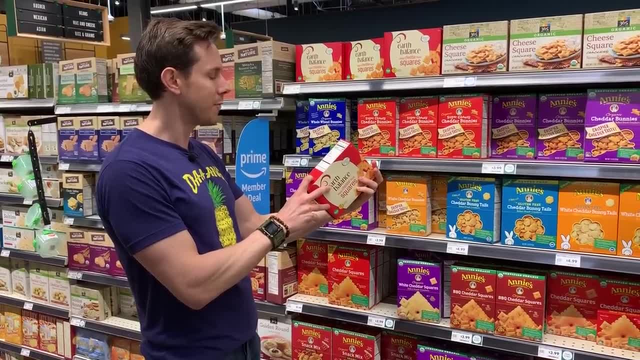 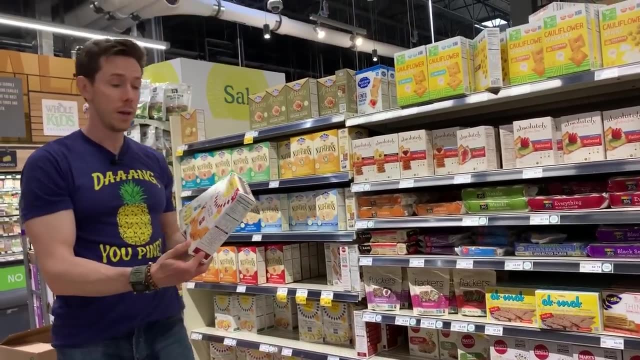 oil. No natural flavorings- Best in class, right here for Annie's. And don't be fooled by the vegan cheddar cheese crackers, because they have a ton of preservatives, natural flavorings, yeast extract and really bad ingredients. Annie's Whole Wheat is where it's at If you guys are looking for a gluten-free paleo cracker. 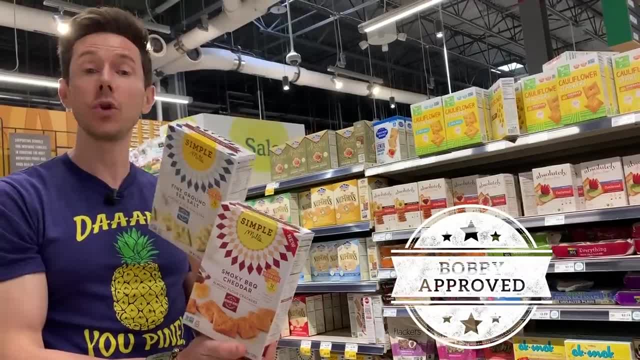 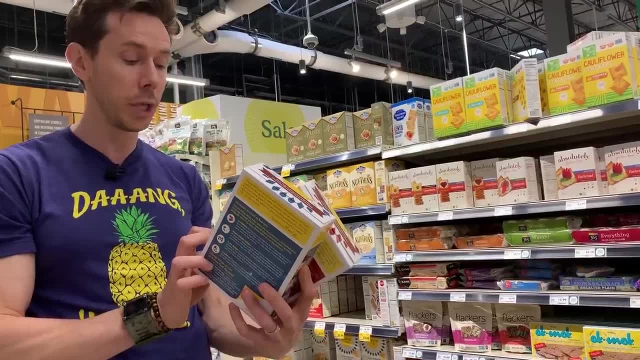 this is best in class at Whole Foods or at Costco The price is way, way better. But look at these ingredients, you guys. Super clean. They're not using natural flavorings or anything nasty, It's all clean. This, my friends, is best in class snacking cheese here at Walmart When we're done. 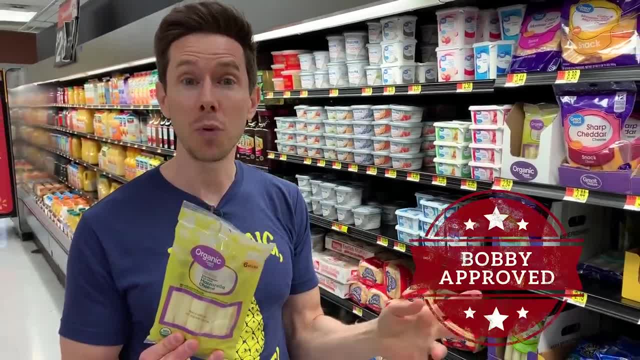 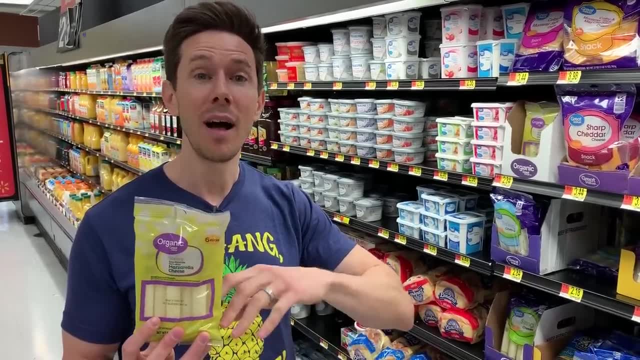 with this video once again. go watch the video for the cheese review. We tell you all about cheese: what to buy, what to avoid and why organic cheese is the best. Organic dairy cows are pasture-raised, grass-fed for at least four months of the years And the 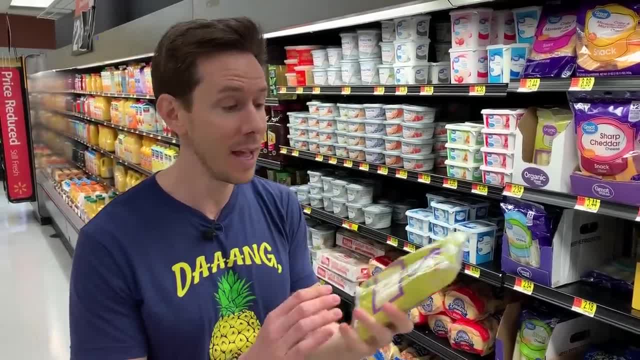 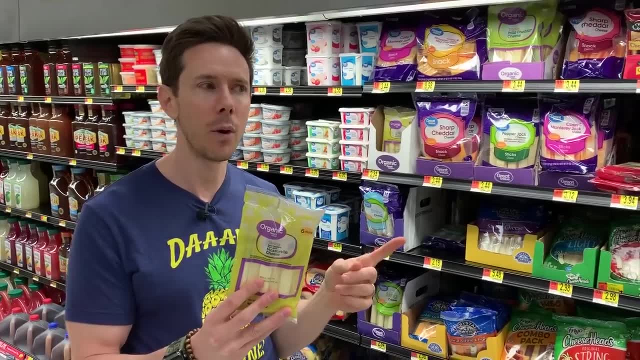 nutritional profile of organic dairy is miles better than conventional. This is great because it's organic string cheese. The price is fantastic. They do also have organic stringles from Organic Valley at Whole Foods, and goat cheese string cheese too. But of all these snacks here, I would 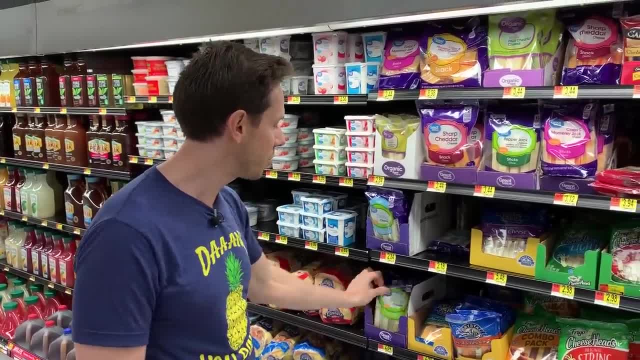 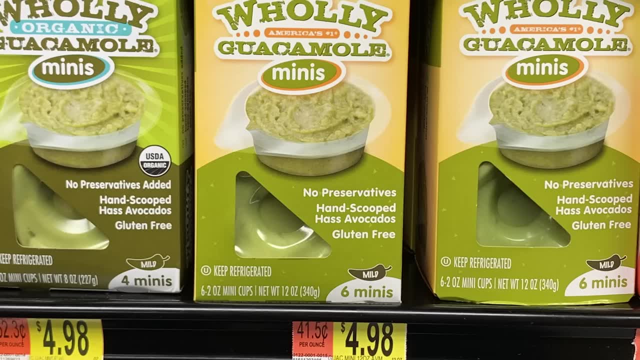 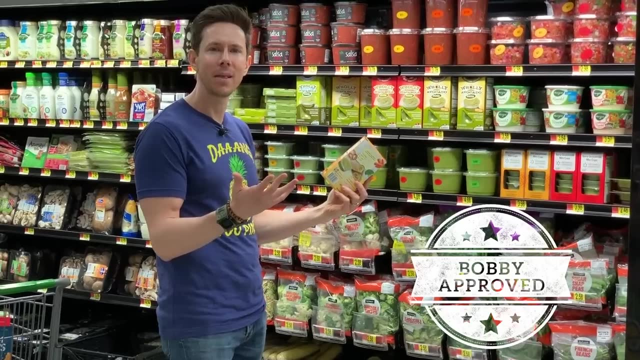 rock this in a heartbeat. This is fantastic for the kids. Conventional dairy string cheese not nearly as good for you as organic. I'm really, really stoked to see something like Holy Guacamole here, because it is tasty and the ingredients are fantastic. I was fully expecting to see something like natural flavorings in here. 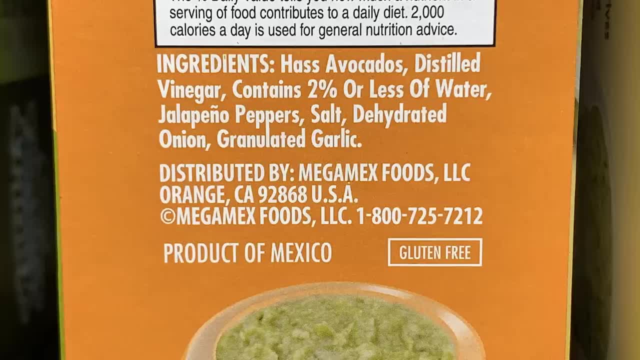 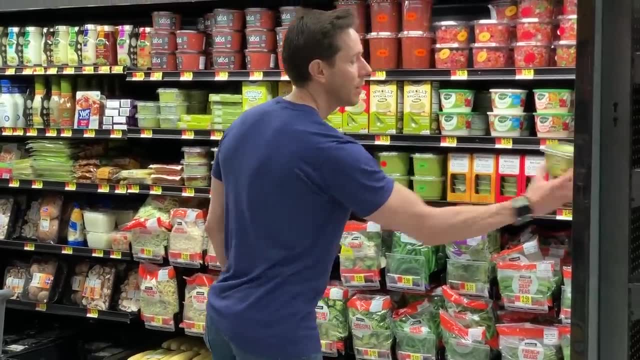 preservatives or something to keep it from turning brown, but they vacuum seal it, so you don't actually have to put preservatives in here And it's super clean. Once again, it's brand Sabra. You compare the ingredients to the Holy Guacamole. There's so many more ingredients here and they're 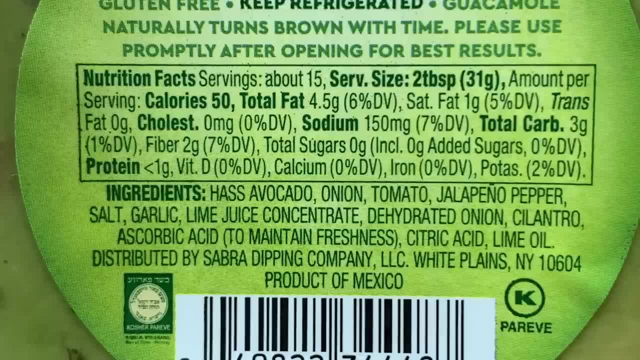 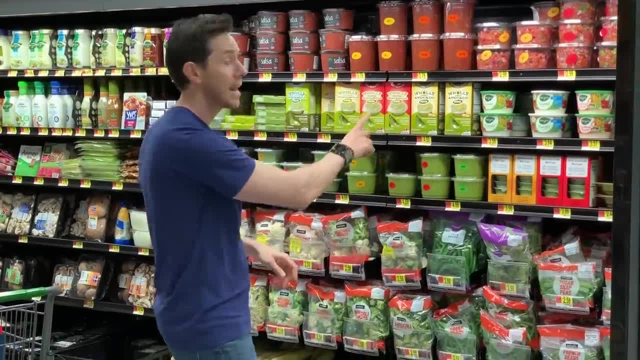 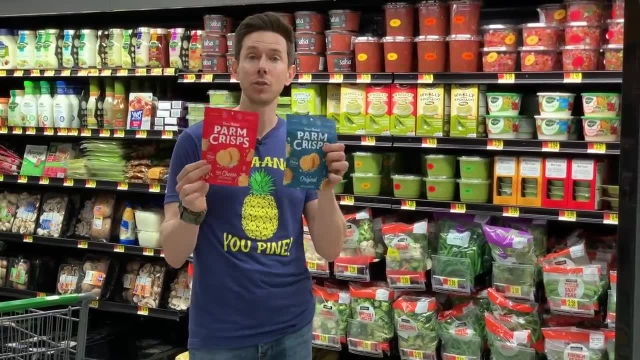 that are super acidic, So I would not get that. I would definitely get that, And if you need something to scoop into there, I just saw these around the corner. These are getting really popular lately. They're cheese crisps made with one ingredient- Parmesan cheese- or four ingredients. 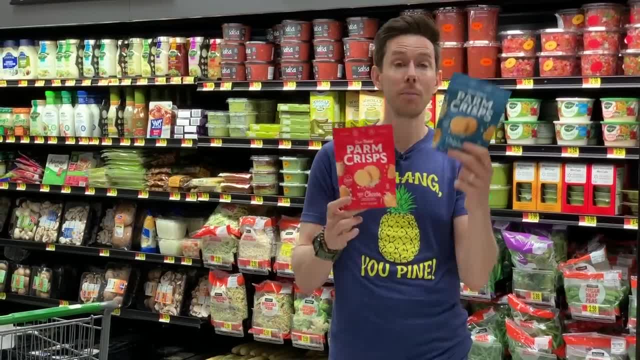 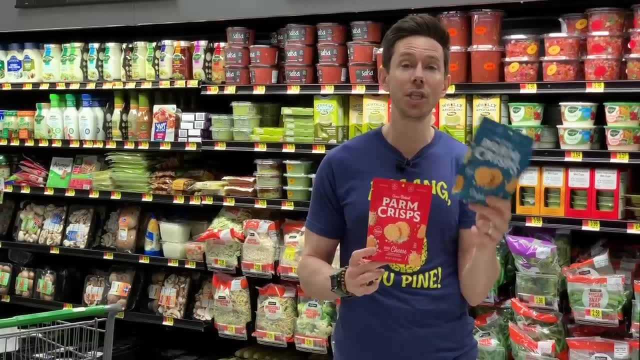 four cheese, Parmesan crisps or cheese crisps. And what I love, especially the Parmesan crisp, is because if you're lactose intolerant or can't handle dairy very well, like kiddies, Parmesan or aged cheeses are the way to go, because a lot of the lactose is eaten. 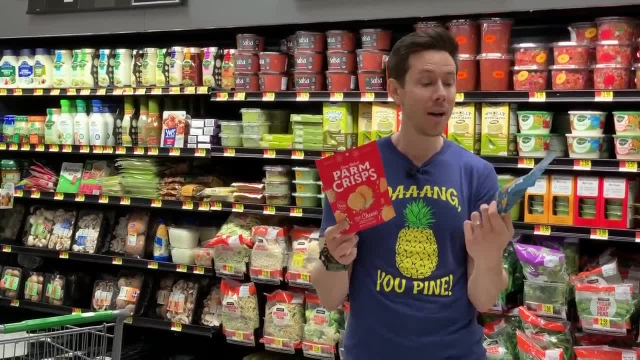 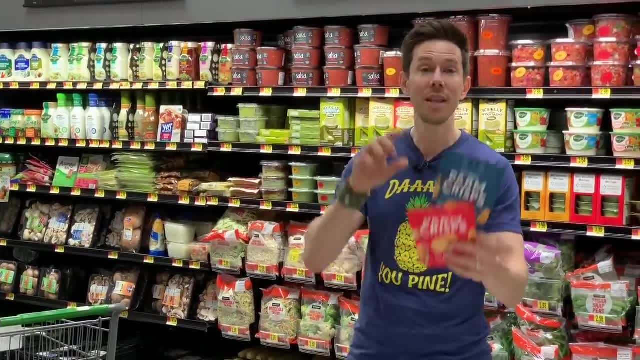 away by the bacteria in the aging process. They're low carb, They're keto friendly and they make a great chip or a crisp to dip into Guacamole or crumble over salads. These are really cool. They have an amazing deal on this at Costco. I would scoop this one all day long. 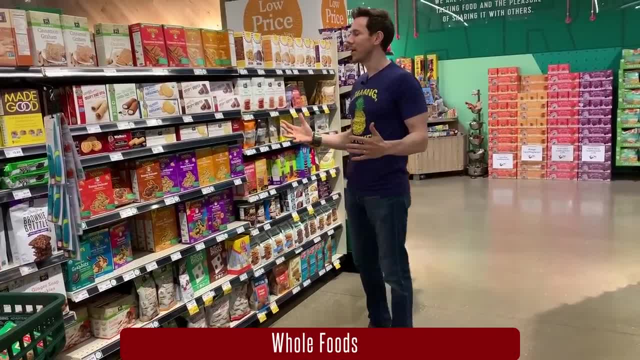 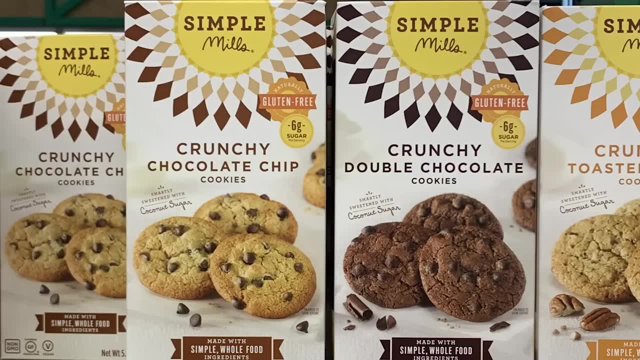 Cookies crackers. I really want to find something here, because I want to believe there's a clean cookie out there, But you guys, I cannot find one anywhere. Case in point: this is a great brand here. It's actually a really good brand. It's a really good brand. It's a really good brand. It's. 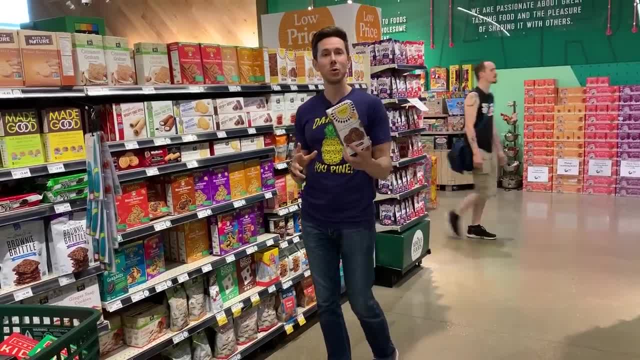 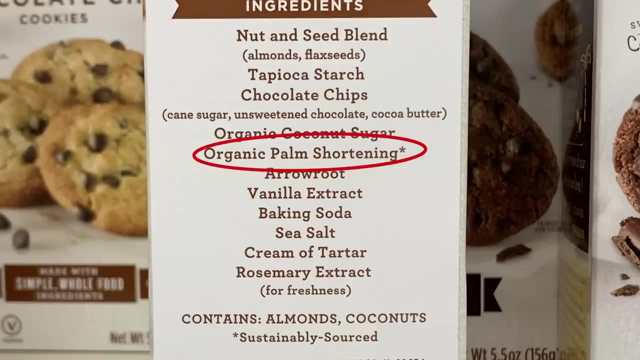 actually based out of Chicago. It's gluten-free. They make fantastic gluten-free crackers. You can actually get them at Costco for a great deal. But all the ingredients here are super, super clean, except for organic palm shortening. You guys, that's palm oil that's been hydrogenated. 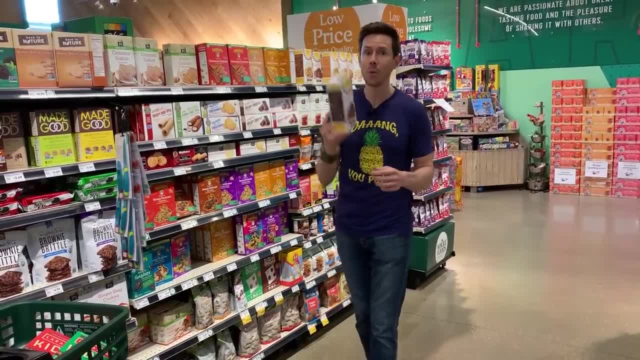 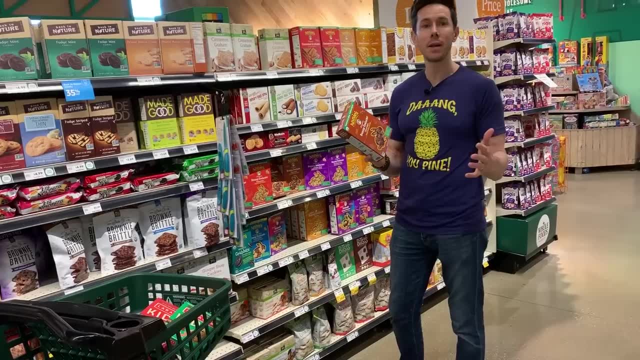 into basically Palm Crisco. This stuff is really bad for you. I would not give that to your kids. Then you look at Annie's. I mean, Annie's disappoints me in some respect And then in other respects, like I'm going to show you with their mac and cheese. 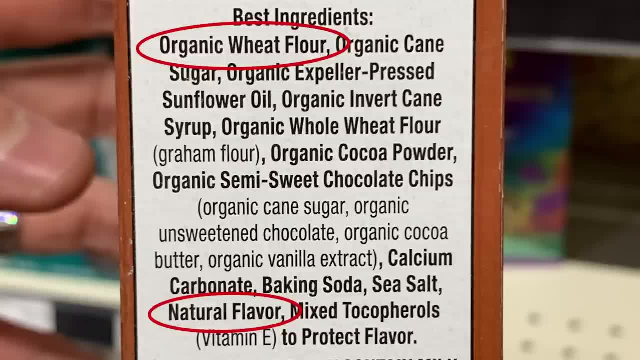 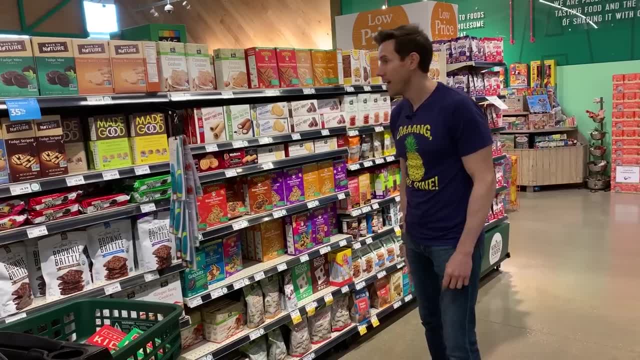 it's amazing They're using organic wheat flour. It's not whole wheat flour, So I'm not a big fan of refined wheat. And then they seem to put natural flavors in a lot of their stuff, So that's a no. And then this brand here makes really good granola, which I'll show you in a minute You can. 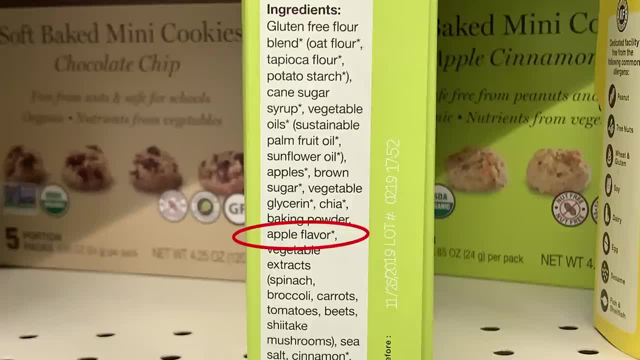 get it at Costco too, But they're tricky here. They put apple flavoring in here. Apple flavoring is another word for natural flavoring, And they're using palm oil and sunflower oil. So that's a no for this one too. 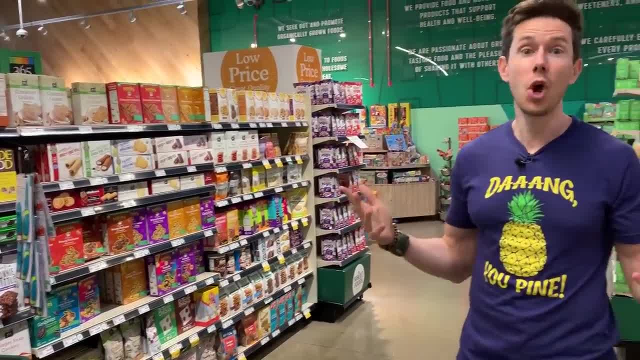 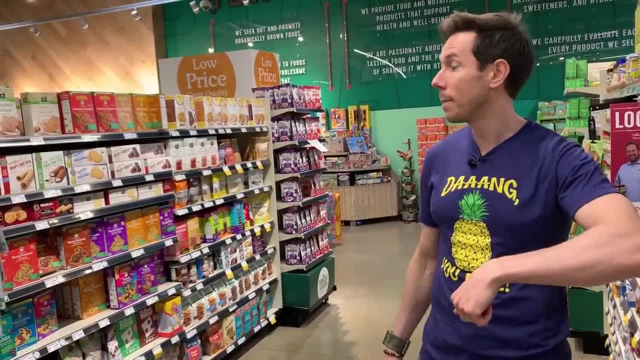 And I just hate to say it, I can't find a cookie here. If you guys know of a really clean cookie that uses real ingredients, no natural flavorings or no bad preservatives, leave a comment down below. But I just saw this on the end cap, So we all know that I really like the Larabars over Waldo. 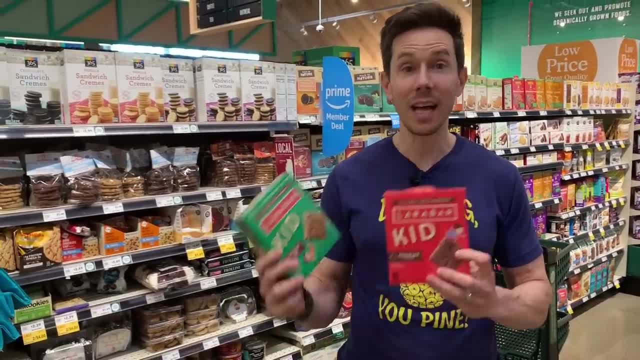 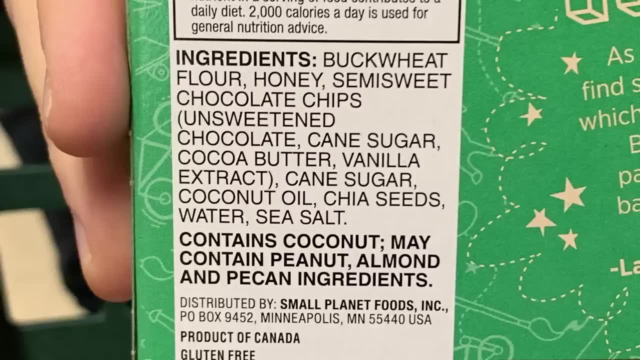 All right, Employees are gone, but it's getting a little crowded in the aisle. Larabar Kids: Super, super clean ingredients. you guys Look at this: Buckwheat flour, honey, real vanilla extract oil. This is not only what you want to feed kids, This is what I want to feed the big kids Baby. 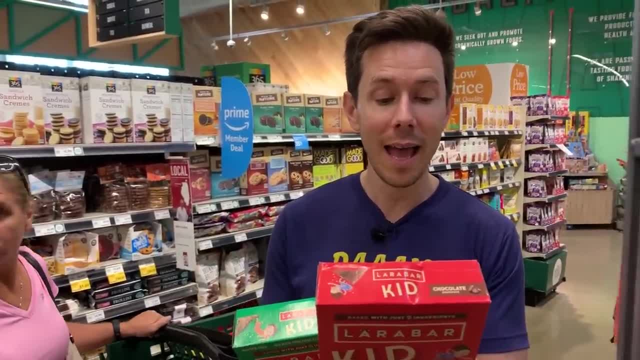 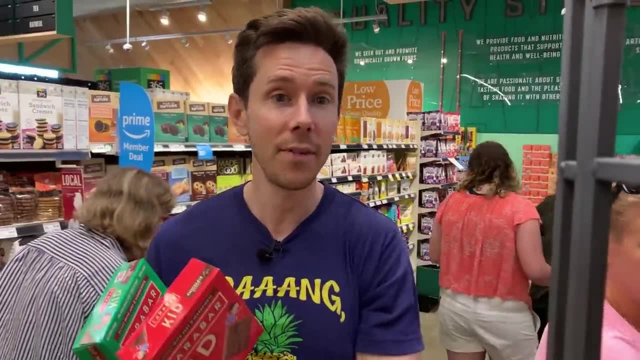 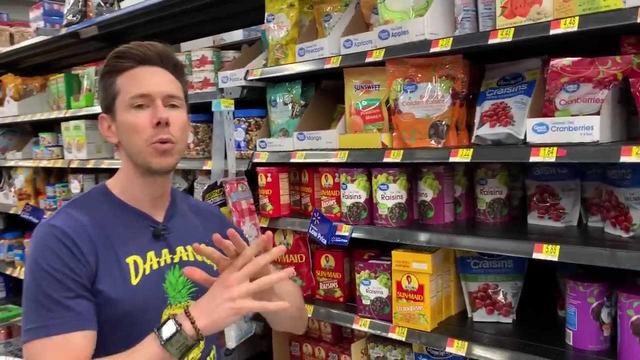 Bobby wants this kind of stuff too. Do you notice how they're not using any kind of natural vanilla flavors, any kind of crappy oils? This is where it's at, Lara, whoever you are, big high five to her. Talk about dried fruit and such Very, very interesting. The rule is just stick with regular. 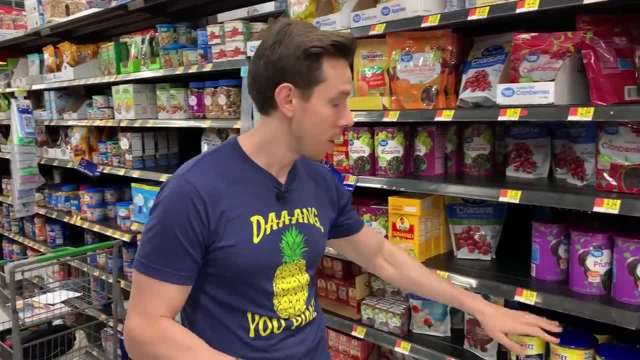 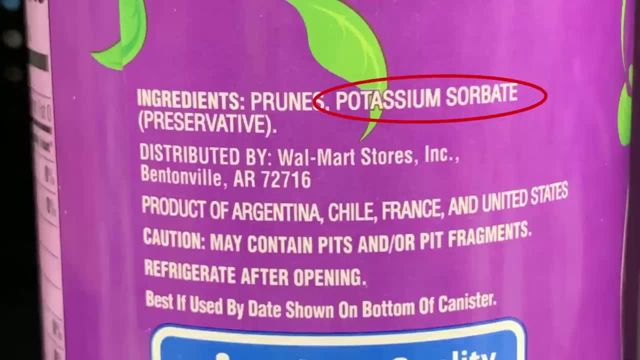 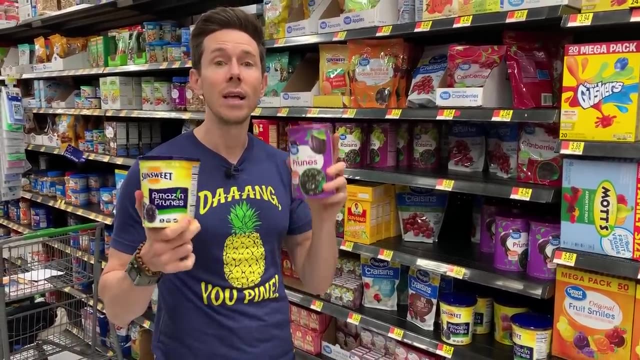 basic dried fruit. But even then there's something troubling about a lot of dried fruits including them. It's always two ingredients: It is prunes and potassium sorbate. Sorbate is a preservative. It's also very bad for your gut and your gut bacteria and your intestines. Some places like 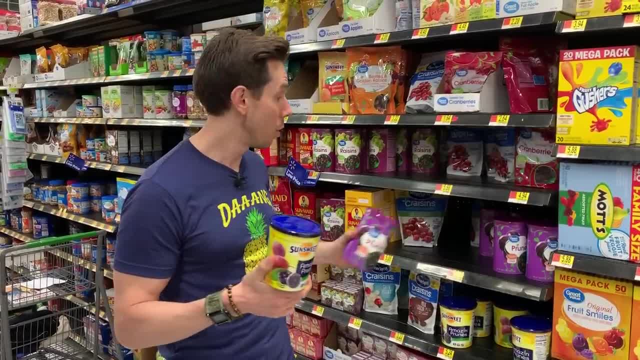 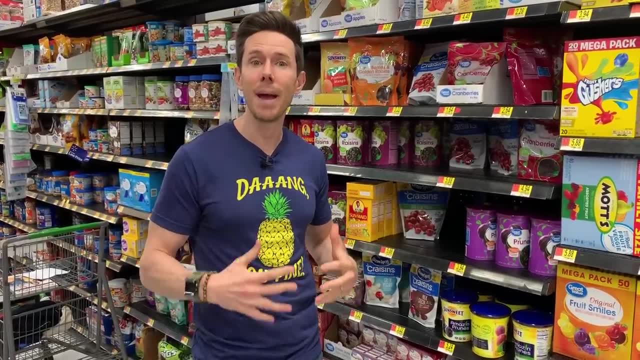 Trader Joe's sell non-sorbate prunes. I would highly recommend buying those because, once again, when you're a child, your microbiome has never been stronger. You have the most amount of living good bacteria in your gut. Foster that Nurture those bacteria. Don't kill them with sugar and 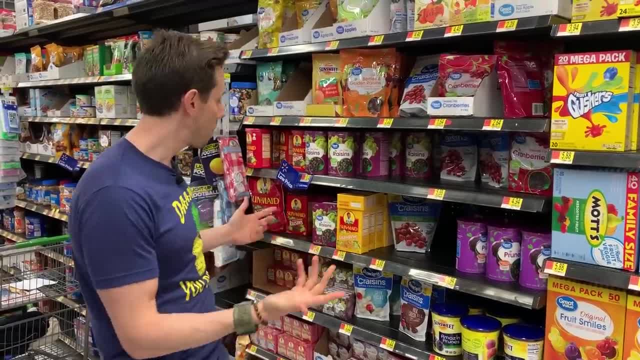 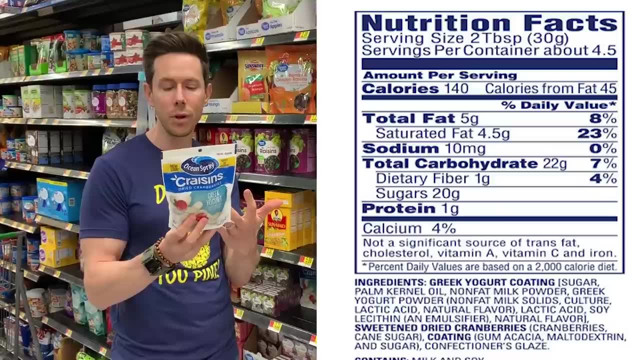 bad foods, because your health is dependent upon your gut, And something you might think like Greek yogurt-coated craisins. Look at the ingredients, you guys. First of all, there's yogurt there, Greek yogurt, which has good probiotics and protein. But 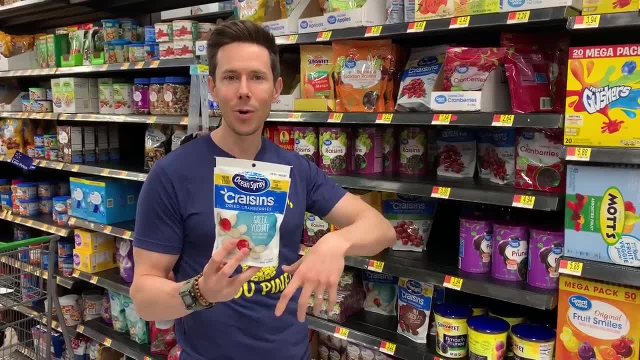 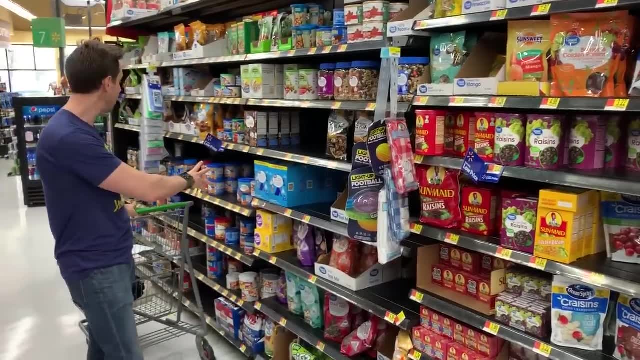 they're combining it with a ton of sugar. When you combine sugar with yogurt probiotic bacteria, you kill all the probiotics. This is just candy. We come down here to nuts and everything. Once again, nuts will almost always have natural flavorings and bad oils if you go with flavored 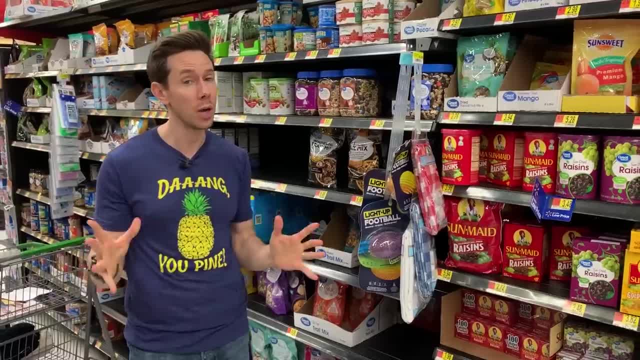 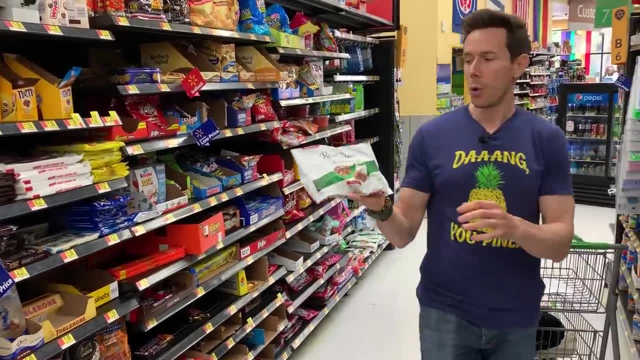 ones Pick ones that have two ingredients: Nuts and salt, or nuts and no salt. That's it. It's super, super easy. A couple people asked me about this on Instagram: Russell Stover sugar-free candies. They're like Bobby, they're delicious. 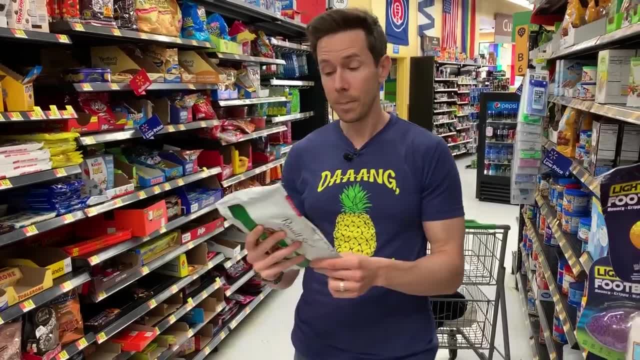 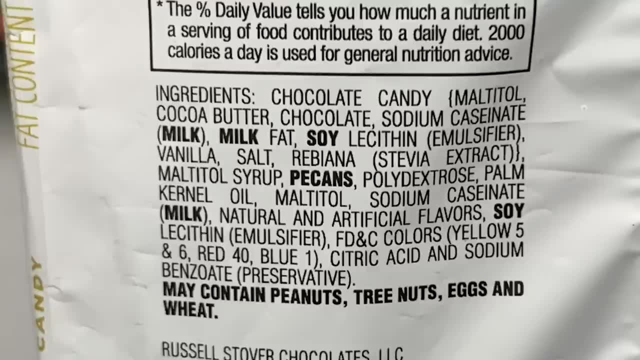 and they're super clean. We're clear. Just look at the ingredients, you guys. All we have to do is read them. There's so many preservatives in here. There's natural flavorings. There's maltitol Two or three times in here, along with natural flavors. Maltitol is going to kill your stomach. 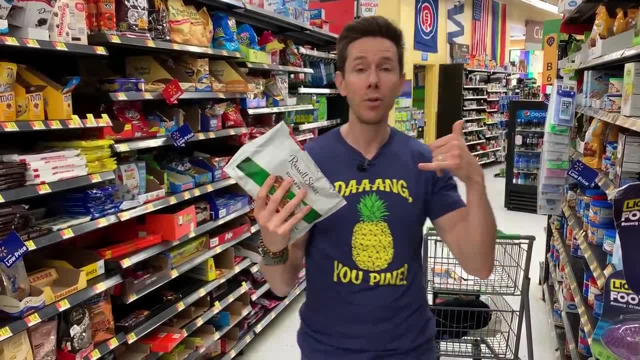 kids, You will poop your pants if you eat this much. You're going to get a call from the principal saying: young Timmy, poop their pants, Pick them up from school right now, all because you gave them this horrible chocolate. Don't do that. 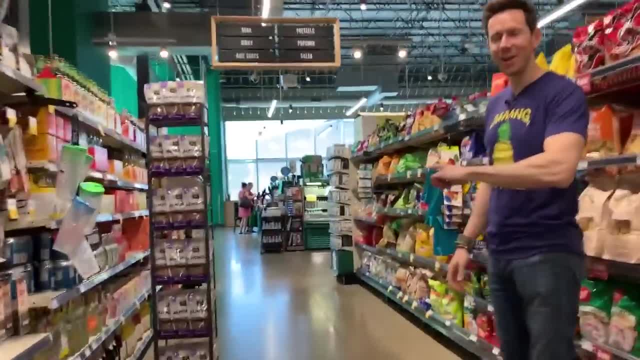 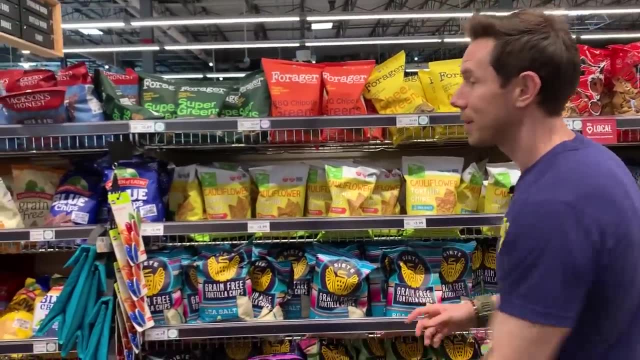 All right, Let's go. The coast is clear. We tried to do this shot now four times, fifth time's. the charm: More chip. we have here. We have a lot more chip varieties here. I want to talk about something that I call marketing misleading. I saw this the other day. They're 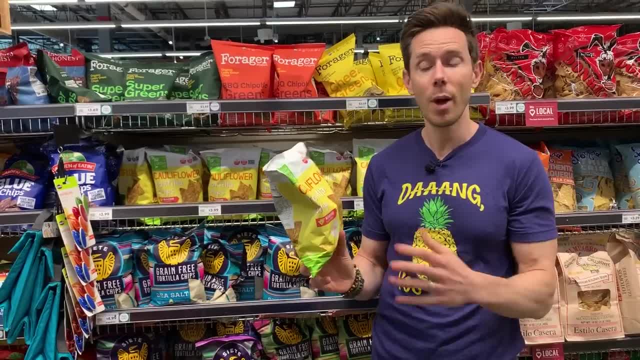 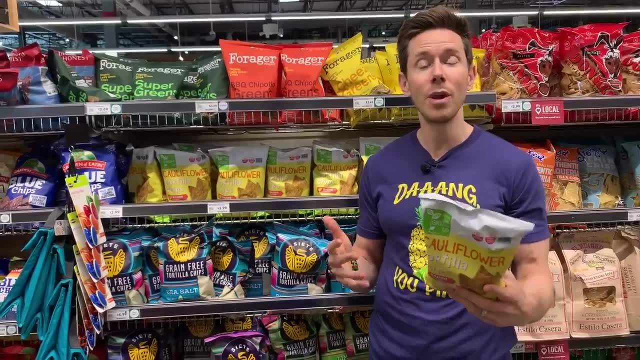 cauliflower tortilla chips, You would expect the first ingredient to be cauliflower. We'll take a look. It's once again cassava starch. Cassava is that South American starchy root vegetable that's relatively cheap. It is grain-free, but don't be putting that as a number one ingredient when 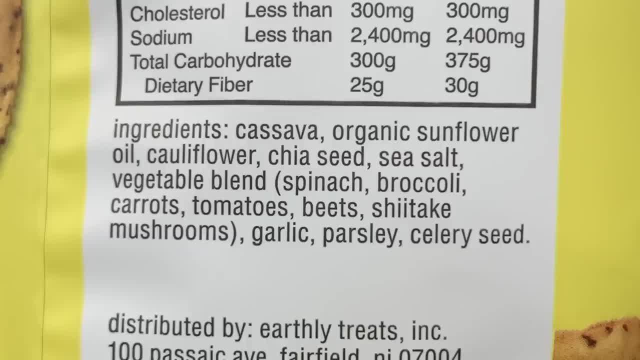 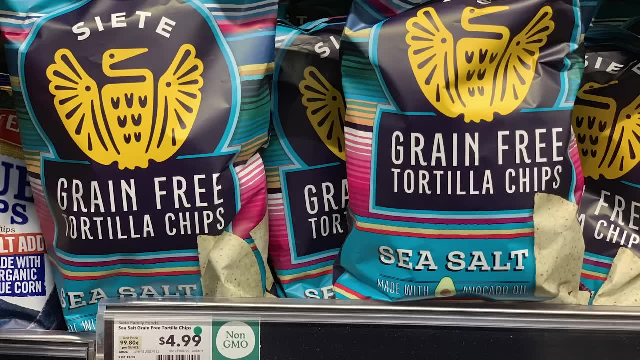 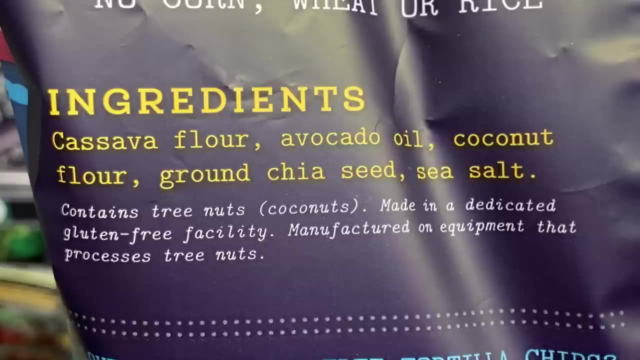 you're calling this cauliflower. It's $4 for a small bag like this. We're talking four ounces. That comes out to $16 a pound. Not cool at all. Siete chips. if you're grain-free or your child is grain-free, this is the perfect chip for you. It's made with really clean ingredients, like 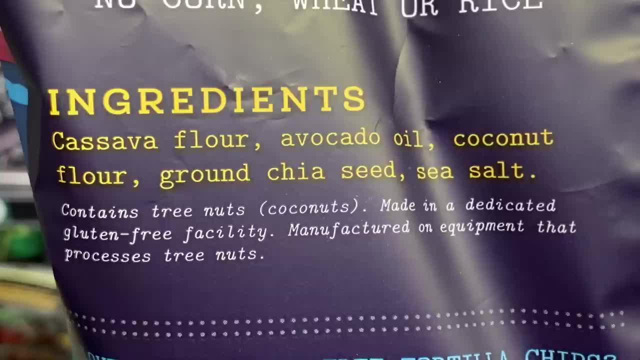 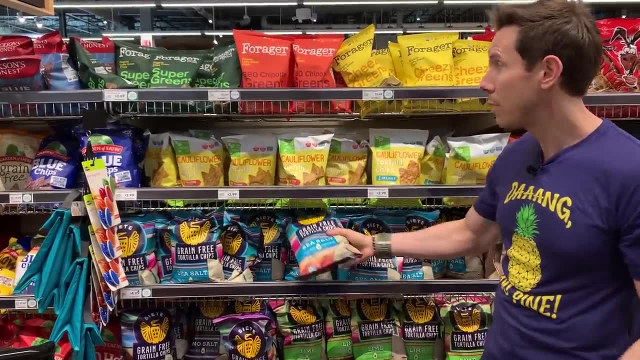 avocado oil and coconut flour. It's made with really clean ingredients like avocado oil and coconut flour. Cassava flour, once again, is the number one ingredient, but they're not advertising that. it's a coconut flour chip. Just keep in mind. it is a starchy, high-carb chip, but it is grain-free. 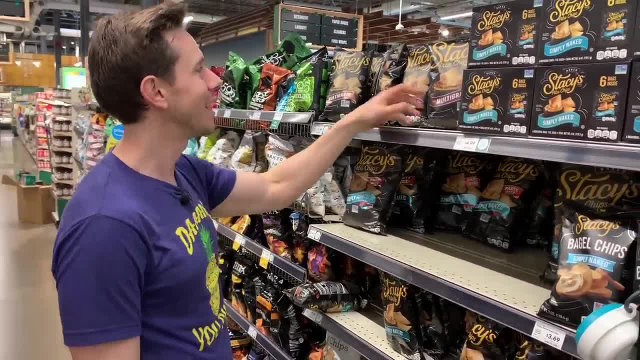 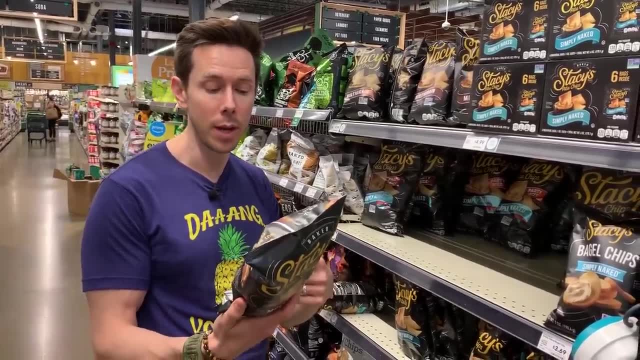 Bobby, is it true that Stacy's mom has got it going on? Well, I don't know. What she doesn't have going on is the fact that I just don't like her chips. I don't like any pita chips, because look at the number one ingredient. 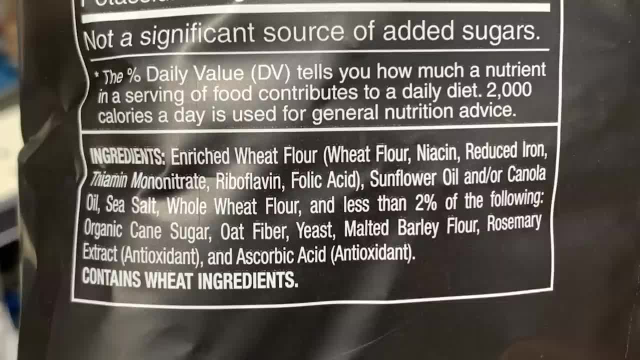 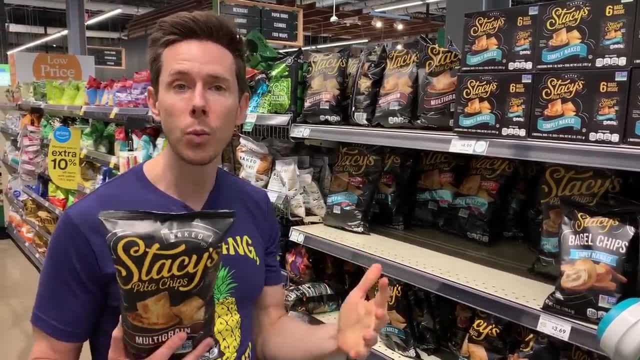 It's enriched wheat flour. I really think it's important for kids and everyone to stay eating whole grains if they're going to eat grains. Enriched flour is just stripping away all the good part of the wheat and only having the endosperm left. That is, the simple carbohydrate. 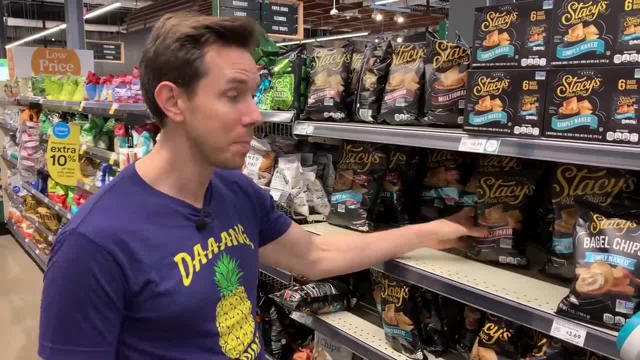 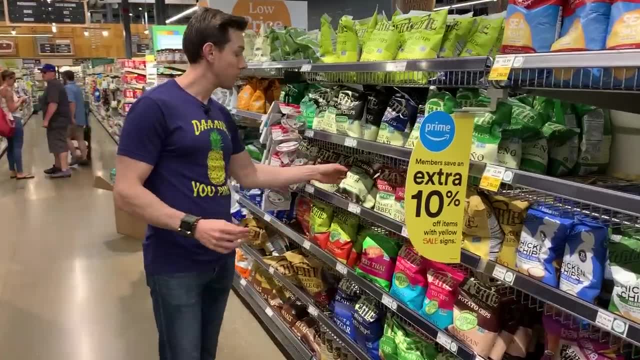 that will spike your blood sugar, which is why I don't like pita chips. You're much better off using a whole grain or some other kind of tortilla chip like the Siete. Ideally, I try to get organic potato chips because potatoes grow on the ground. They're very susceptible to chemicals and 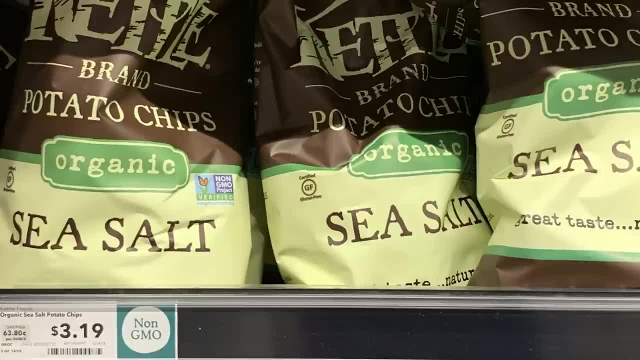 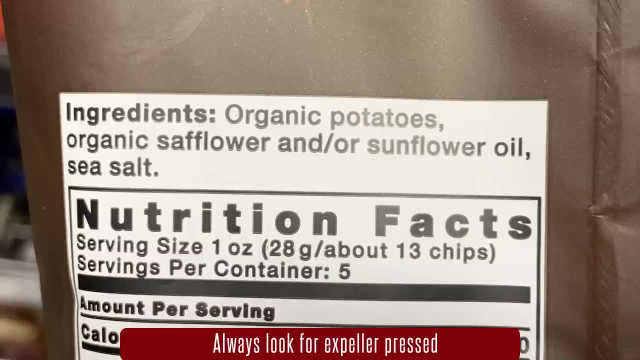 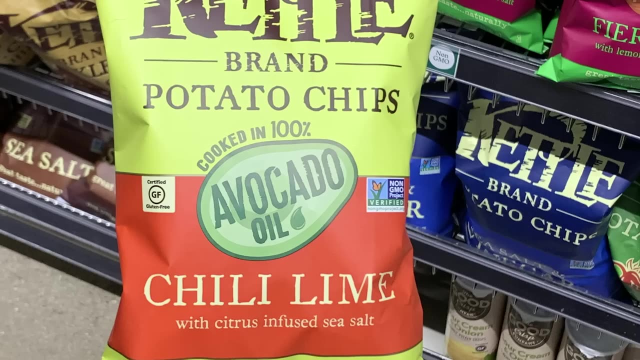 pesticides. Here's a kettle organic potato chip, but it's a double-edged sword, because even though they're using organic potatoes, they're frying it in organic safflower or sunflower oil. It's not kind of a bummer? Then I go to these kettle ones that are cooked in avocado oil. here It's not. 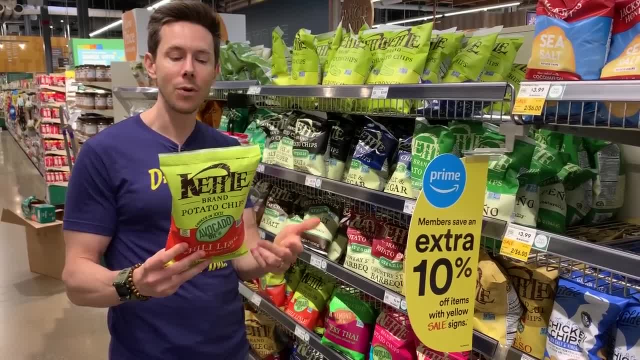 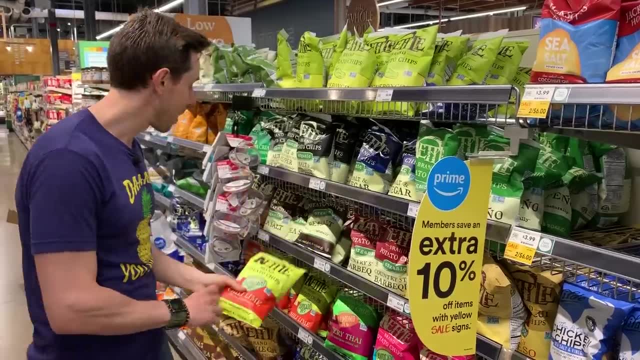 organic, but it is avocado oil, which is very good. Then, because it's flavored, they're using natural flavorings and a couple other things like maltodextrin, which is that preservative that I just don't like. If you're going to go for the avocado oil one, this one, just a straight up. 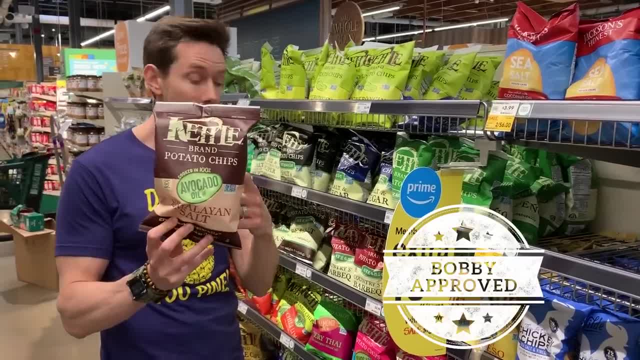 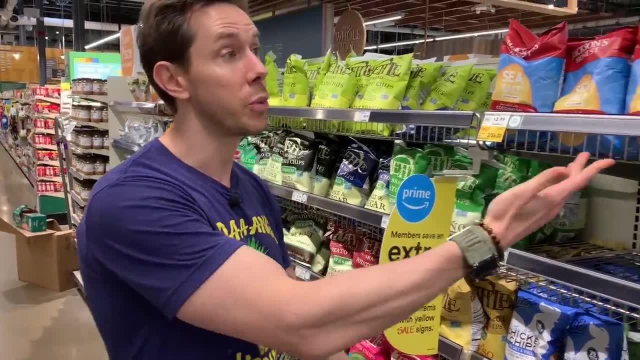 potato, avocado oil and sea salt. This is a really good one, Even though it's not organic. I'd rather get this over the organic one that's cooked in the crappy canola oil. This brand is really good here. Jackson's. 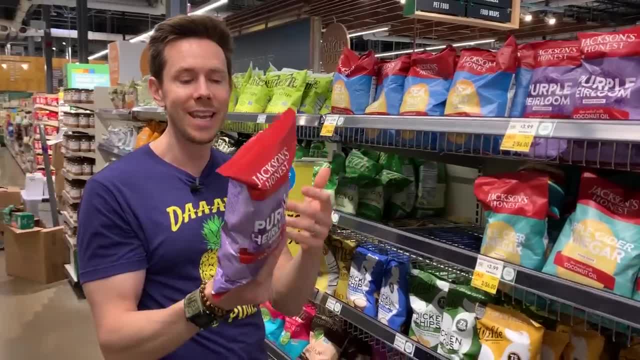 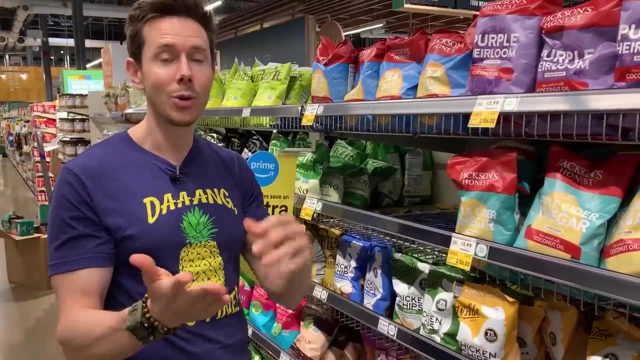 These are purple heirloom potato chips, slow cooked in organic coconut oil. Those are my top two choices, but it's very tricky, because either it's not organic and it's good oil, or it's good oil and it's not organic. Then I see two more popcorns here that are way better than what we talked about. 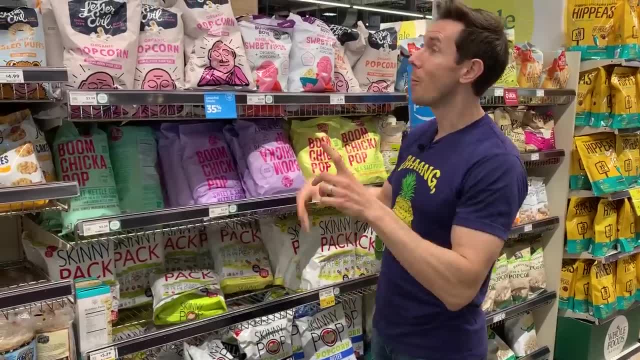 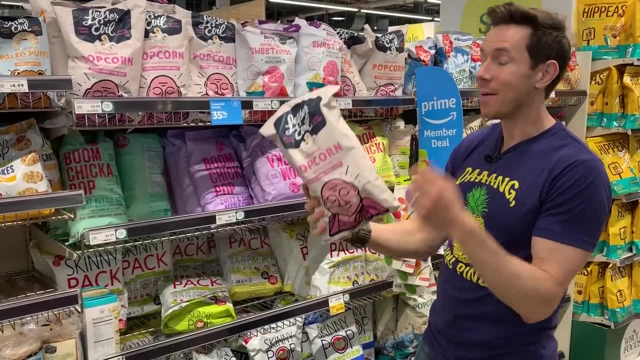 Skinny Pop, which you want to stay away from because they use bad oil. So many of you guys on Instagram have been sending me pictures of this brand. I love that name. This is amazing. Look at the ingredients. organic, non-GMO popcorn. 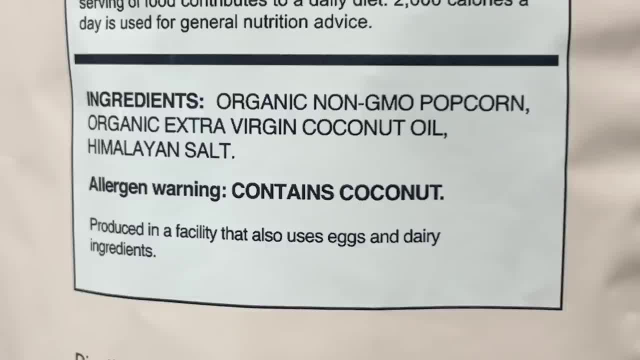 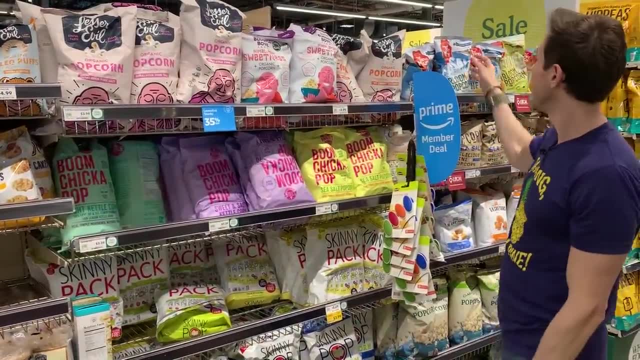 organic extra virgin coconut oil in Himalayan pink salt Dude. high five Buddha. That is awesome, Namaste. Let's stick to the plain one, because the flavored ones start having natural flavorings. This is a cool brand out of the Midwest. Tiny But Mighty, It's an heirloom variety of popcorn. 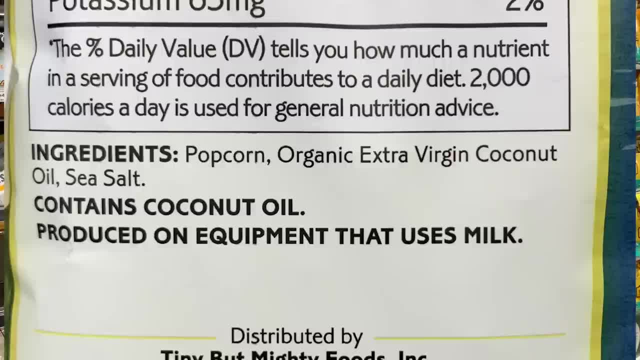 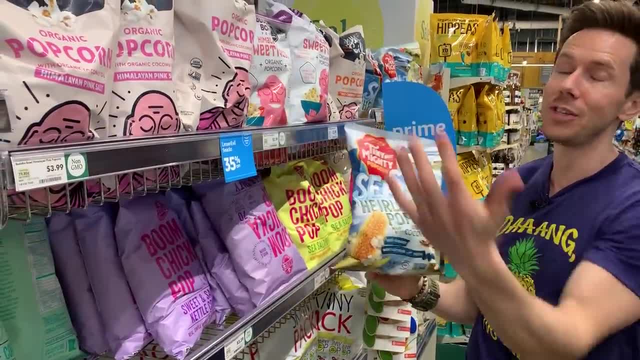 which is easier for your body to digest. It's also cooked in extra virgin coconut oil and it's non-GMO. If I had to choose one, I'd choose a little booty here, because he's just so darn cute, But these are starting to get to really cool popcorn options way better than the. 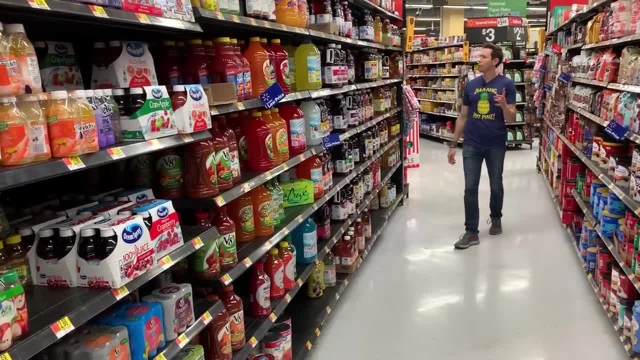 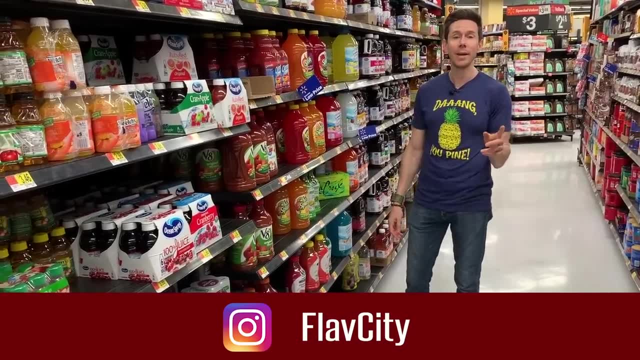 crappy skinny pop Juices were obviously a popular choice on FlavCity Instagram- which, by the way, if you're not following me, go over there because we do stories of what we're making for dinner every night and it's a lot of fun. The thing is, you guys, I don't see one. 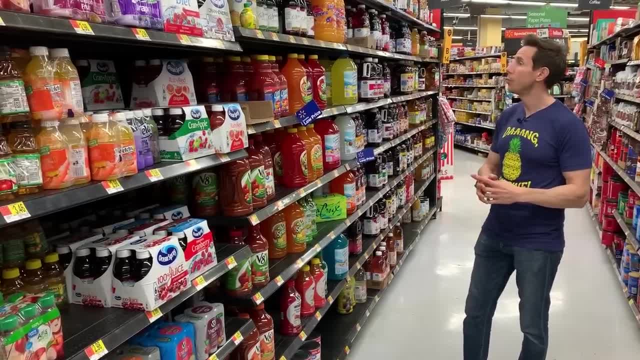 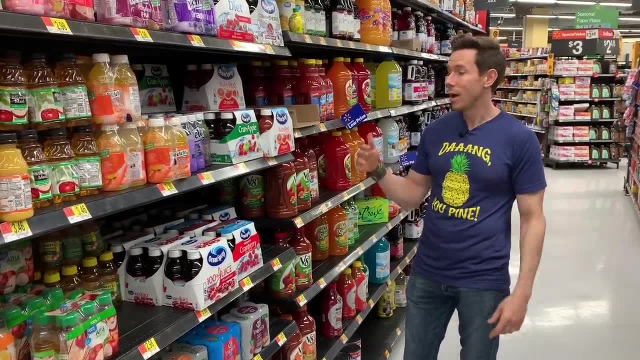 juice I can recommend, at least here at Walmart, maybe at Whole Foods later on. All these are either highly processed, highly pasteurized. you kill all the good nutrients in there, have sugar or natural flavors, even something that's basic. This is not a juice, but this is. 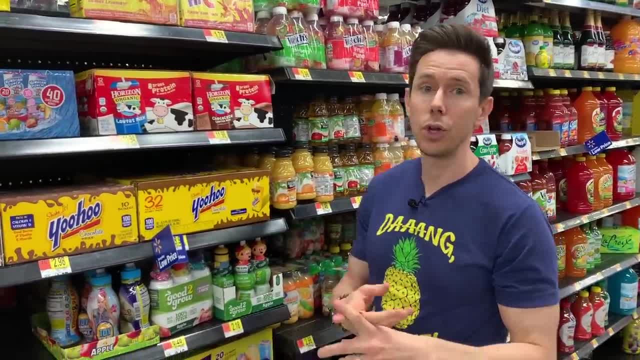 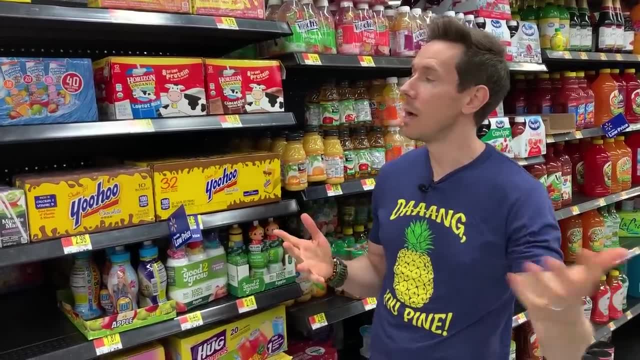 shelf-stable milk. If you're wondering how they make it shelf-stable, it's called UHT- ultra high temperature pasteurization. While it does kill a lot pretty much all the living organisms or enzymes in there, it's still better than this because it's lower in sugar. 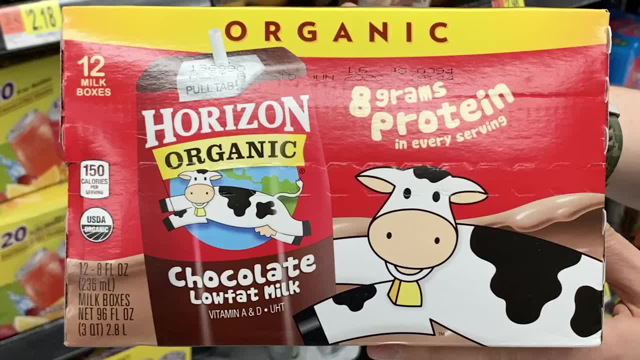 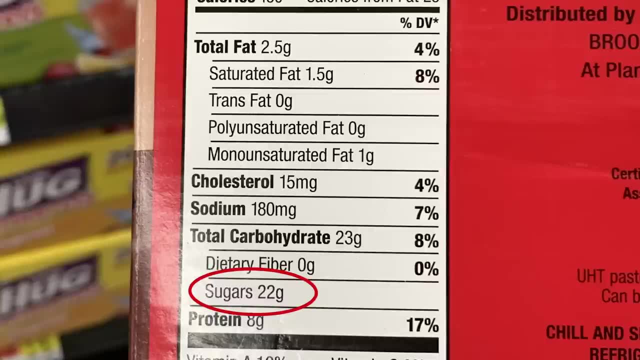 has more protein. but stay away from chocolate milk, you guys. Any kind of chocolate milk or non-dairy milk Has scary amounts of sugar We're talking about. one eight-ounce fluid box has 22 grams of sugar. You guys, there's four grams of sugar in a teaspoon. Imagine little Timmy or little Erica. 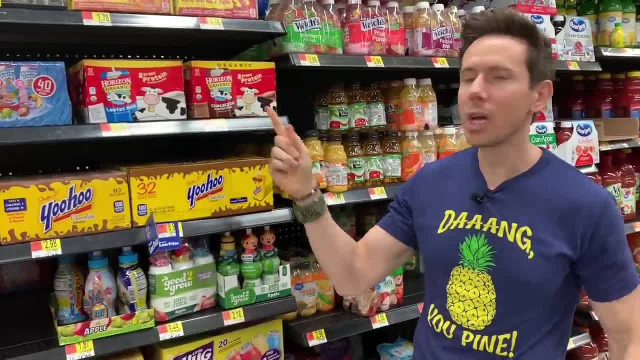 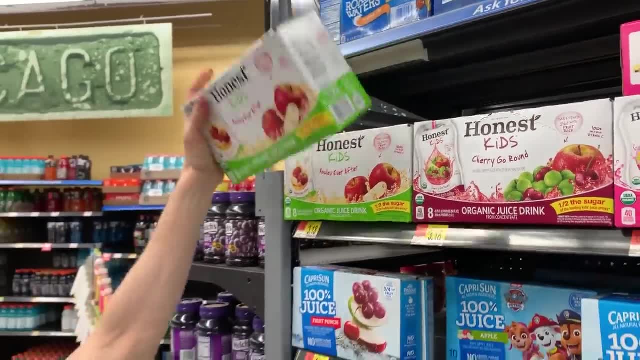 getting over five teaspoons of sugar. They're going to be bouncing off the walls. It's totally nutball. Then wait a second. I did spy this out of the corner of my eye. Honest is a good brand, but you might think it's going to be clean, because the brand is trustworthy, You guys. 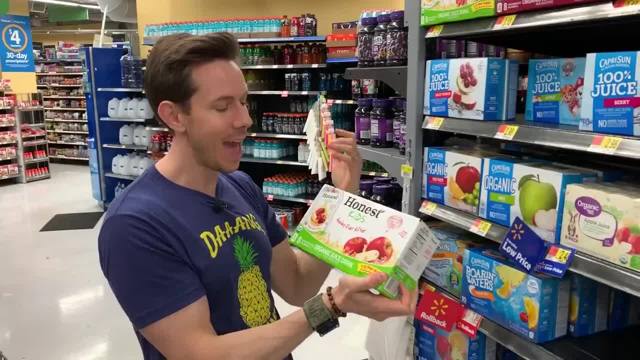 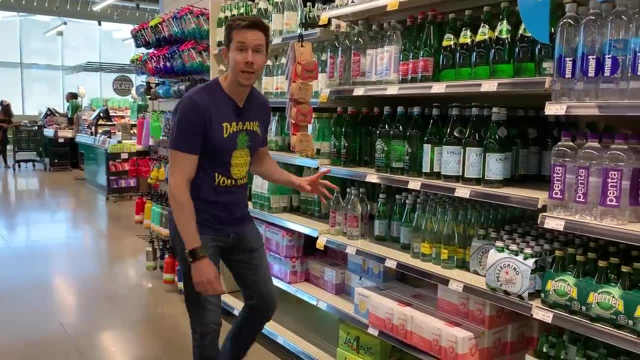 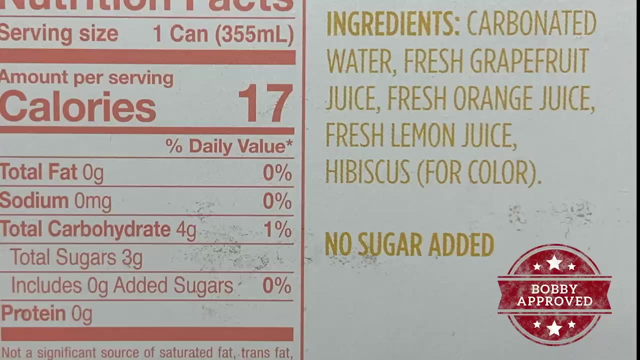 look at the ingredients: Natural flavorings even in apple juice. That is super, super sad. Like I said, there is not one juice here that I can recommend. One of the only flavored sparkling waters I can find anywhere without natural flavors is Spindrift. It literally is just the real fruit water. maybe some lemon juice Every. 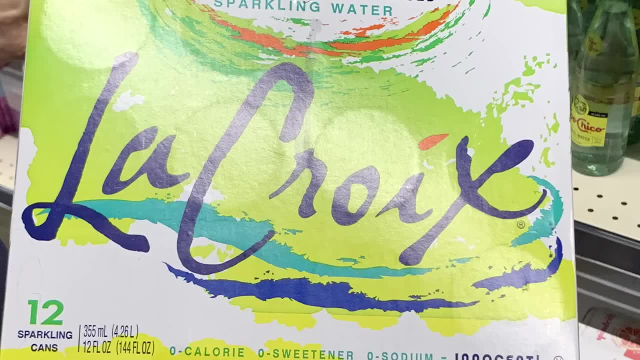 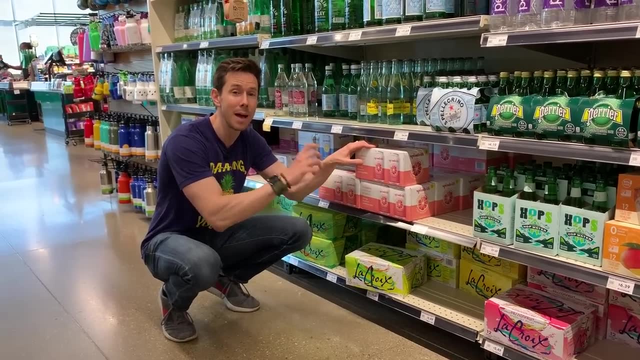 other flavored drink, especially LaCroix, has natural flavorings. LaCroix is ballsy enough to actually call it natural essences, which is total a crock. but this stuff is the real deal. I love it. You can buy it by the can at Trader Joe's too. 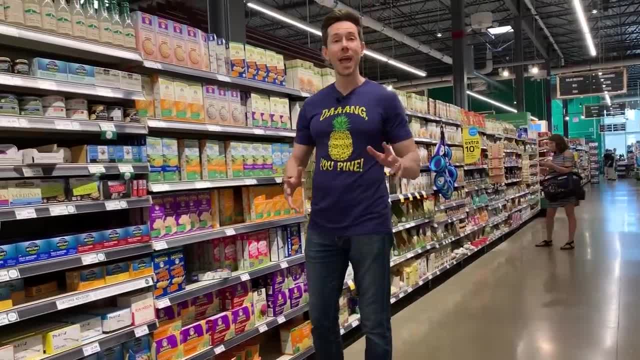 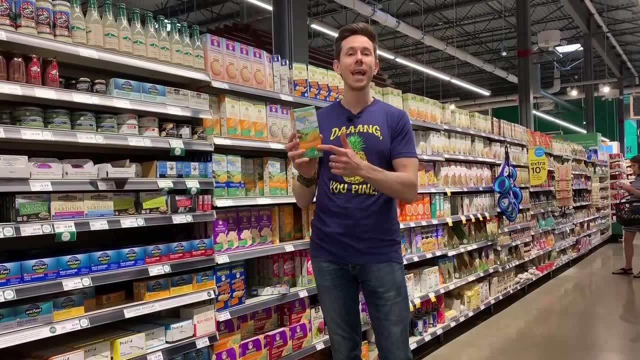 Are you guys ready for the best in class mac and cheese you could ever feed your family? It comes from Annie's. She's totally redeemed herself from the gummies we saw earlier. It's organic grass-fed mac and cheese. Grass-fed dairy is where it's at. It has the highest nutritional profile of any other. 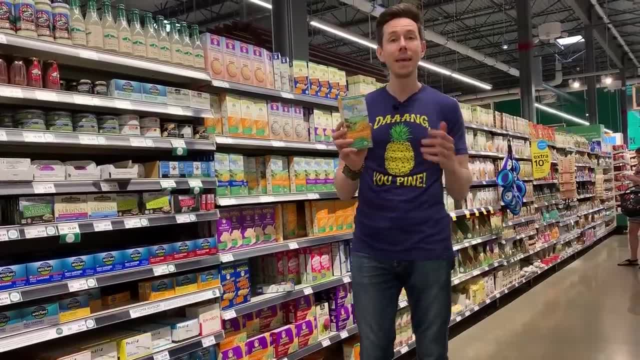 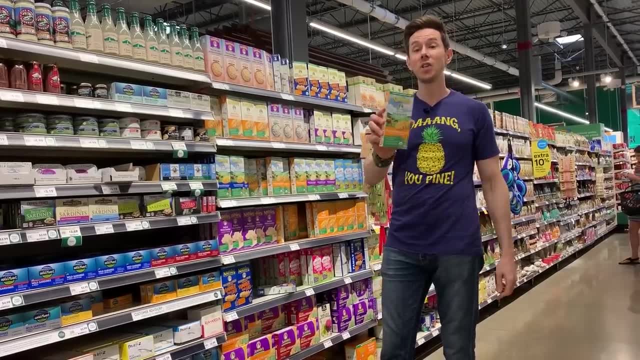 dairy. I've never seen any other brand anywhere else make organic mac and cheese from organic dairy. It comes in three flavors. It's a little pricey but if you can afford this, this is the only mac and cheese I would feed my kids. That is amazing. 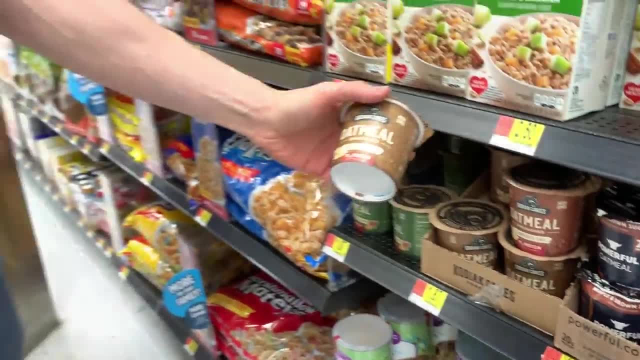 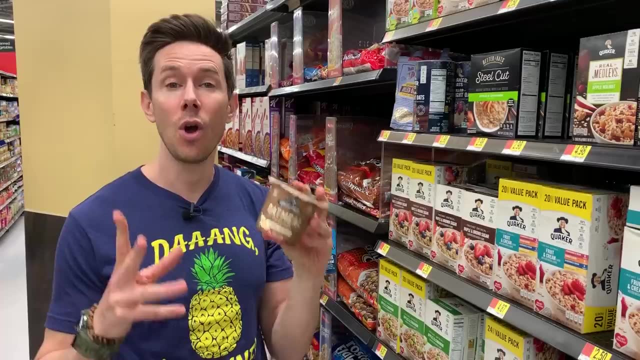 This caught my attention out of the corner of my eye. You might want to give your kids oatmeal in the morning for breakfast. Kodiak Cakes is a very popular brand. The thing is, when you're giving oats to kids or in general, always get organic oats, because conventional oats are often sprayed. 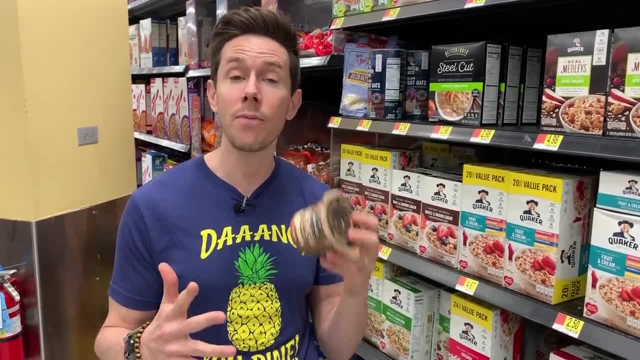 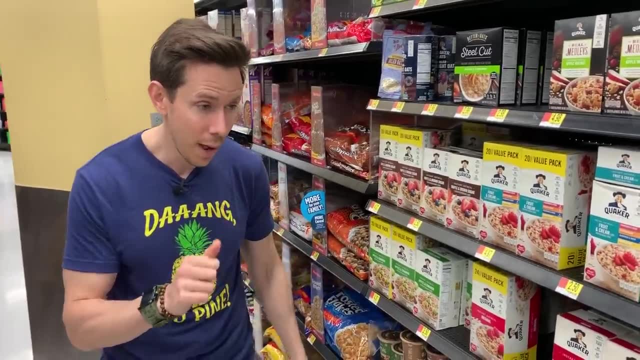 with glyphosate. Glyphosate is the active ingredient in Roundup from Monsanto. Super, super bad news. I don't see any organic oatmeal here. I'm pretty sure they're going to have it over at Whole Foods. It's something I just wanted to let you know. You know what I caught? this. 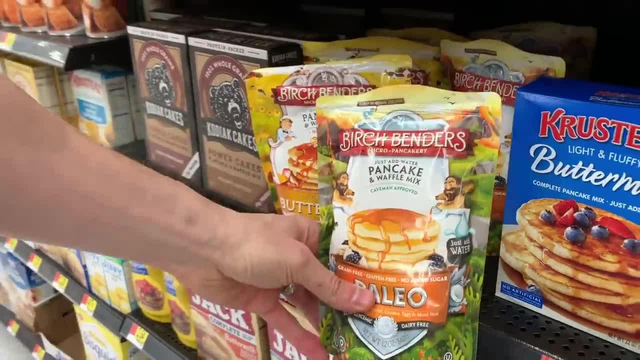 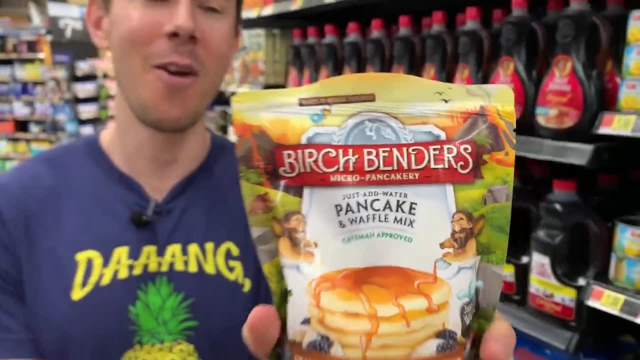 out of the corner of my eye too. It's this stuff, Birch Benders. I get a lot of requests for this on Instagram. First of all, look at Art, and I just saw here Micro Pancakery. This is a first. you. 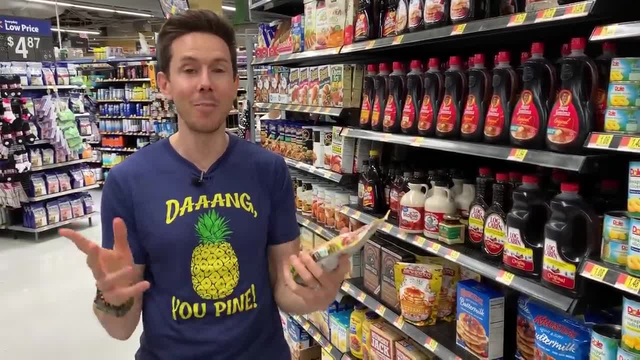 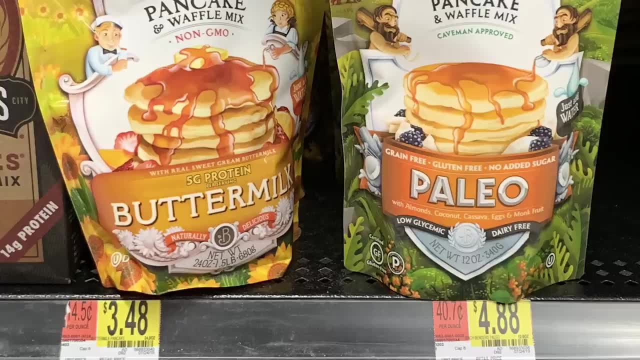 guys. I've heard of micro breweries, but a micro pancakery is a little much. Here's my beef with companies like this. You're charging a premium price for Paleo- $4.88 here- but you're using cheap ingredients. What do I mean by that? The number one ingredient here is cassava starch. 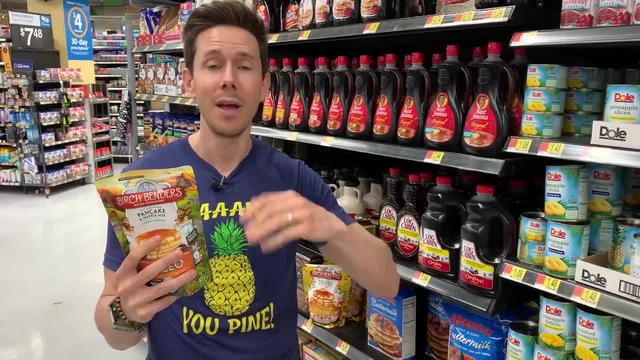 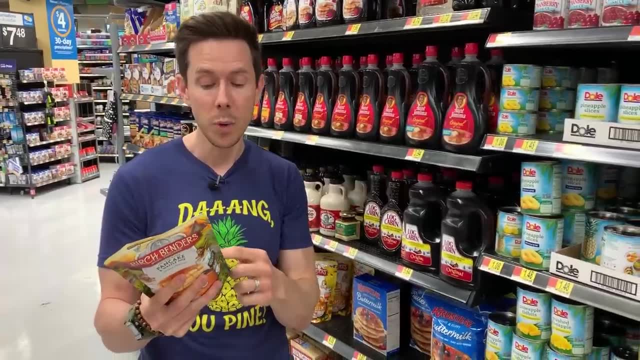 Cassava starch is a cheap starchy root vegetable from South America. It's a very, very, very. on top of that, it's also very high in carbs and simple carbohydrates that spike your blood sugar. Then, two ingredients later is the almond flour. I would much rather almond flour be number. 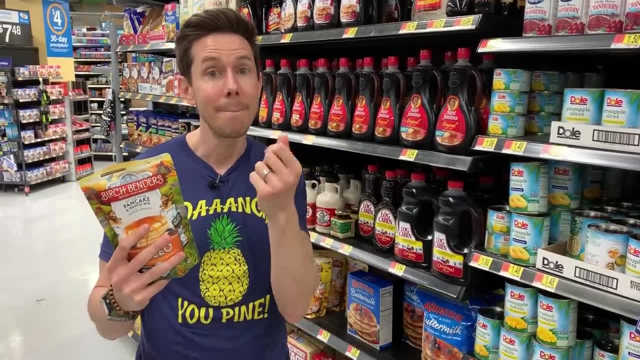 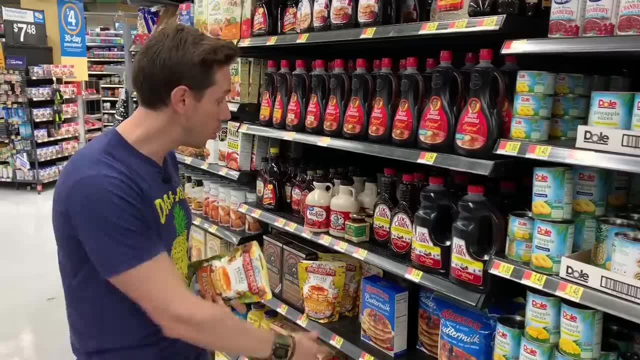 one and cassava be much, much lower. The reason they're doing that Money right. What does Mr Wonderful say on Shark Tank? It's all about money. Stop using the cheap filler and charging me and you the premium prices. That ain't cool. That ain't cool at all. Before we leave this aisle: 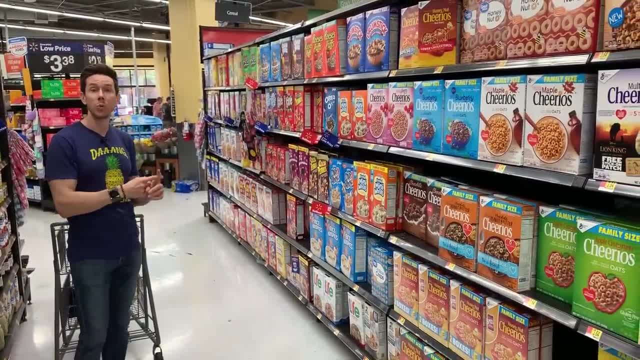 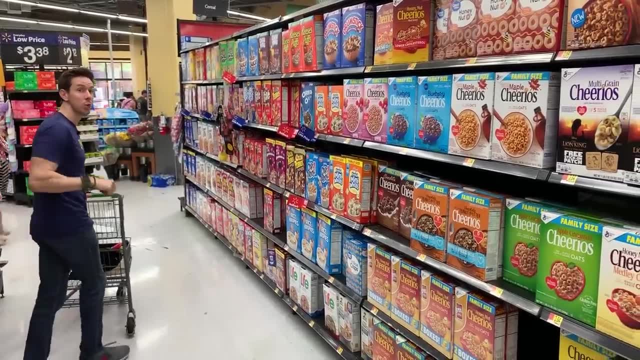 if you want to know what cereal to feed your kids, watch our cereal review. we go deep into cereal. Spoiler alert: 90% of these are just sugary, starchy messes, but there are some really good ones to feed your kids. This- you guys- is maybe one of the most. 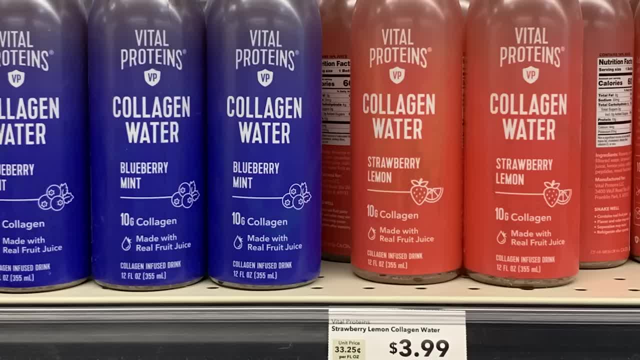 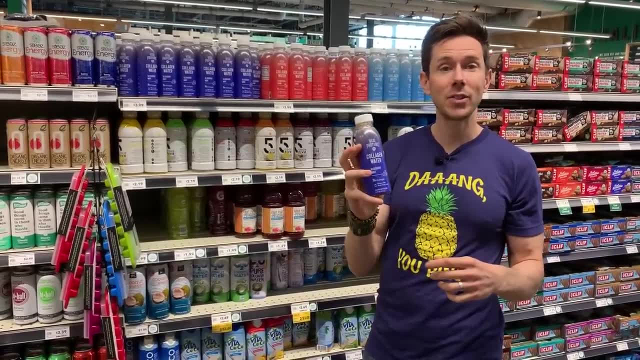 exciting drinks I've seen in a long time. It's Vital Proteins, Collagen Water Once again. whereas your kids might not need it, you might need it because, once again, as you get older, your collagen goes away. This is a great supplement. They have flavors: blueberry, mint, strawberry, lemon. How do 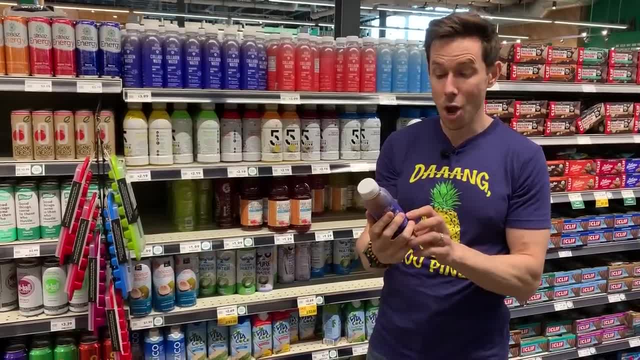 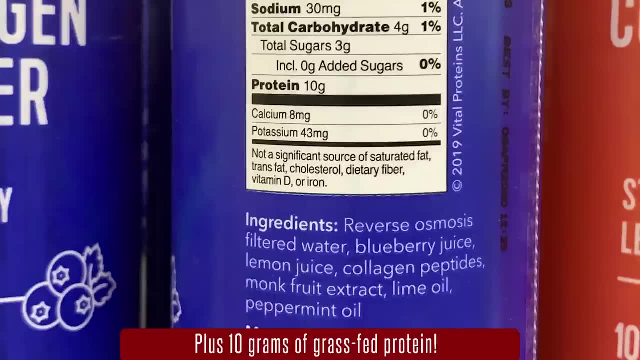 they get those in there. Natural flavors, other nasty stuff, right? No, With blueberry juice, with lemon juice, with monk fruit extract, lime oil and peppermint oil, zero added sugars. This is one of the coolest things I've seen to help you keep cool this summer. They have it now at Costco. 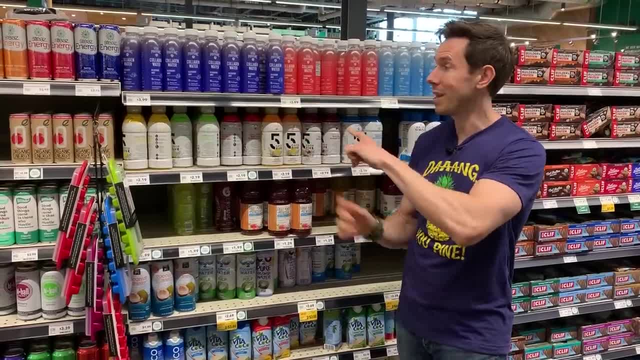 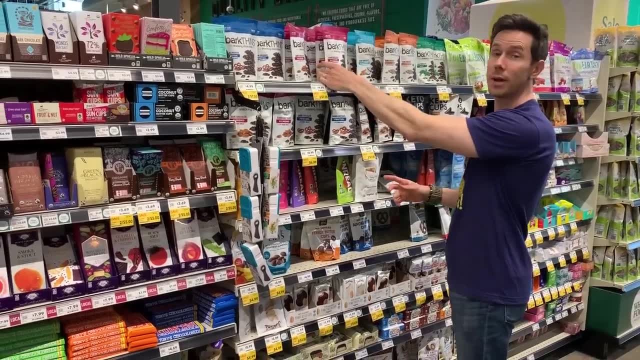 in variety packs. Either way, your kid should drink it. You should drink it. It's a little pricey, but, wow, The best drink in the grocery store right now is that I can't leave this aisle without talking about my favorite snacking, chocolate. Don't buy it here. They have a huge. 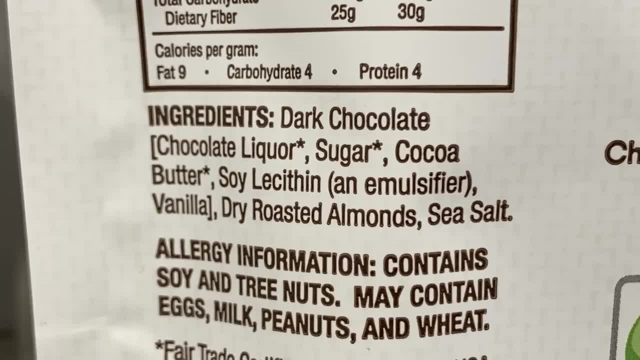 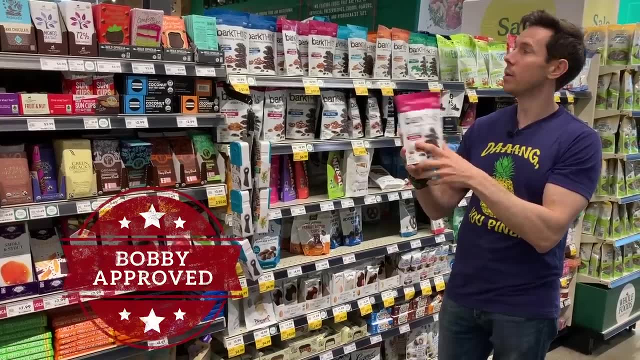 bag at Costco, but Bark Thins. Look at the ingredients. It's just chocolate and the almonds a little bit of soy lecithin, Totally fine, unless you can't have soy Stick to the almond, Don't start going to the pretzel ones. This for a great snack is fantastic for you or for. 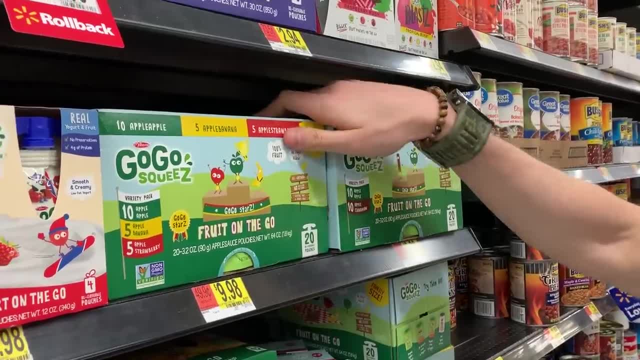 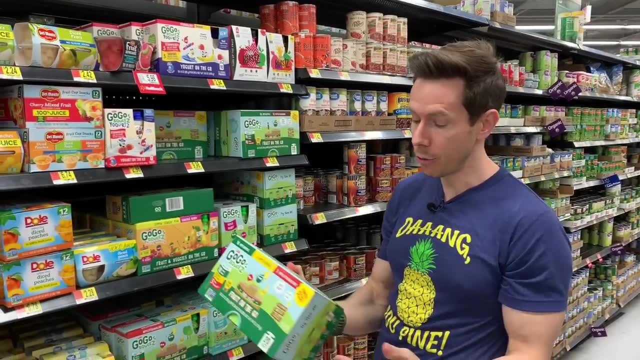 the kids and it's super duper clean. Now, this is a product that I fully expected not to endorse because it seems like something that's wrong. There's fruits and vegetables in a pouch here, but I love the ingredients here. You guys, it's pure fruits and vegetables. There's no added.